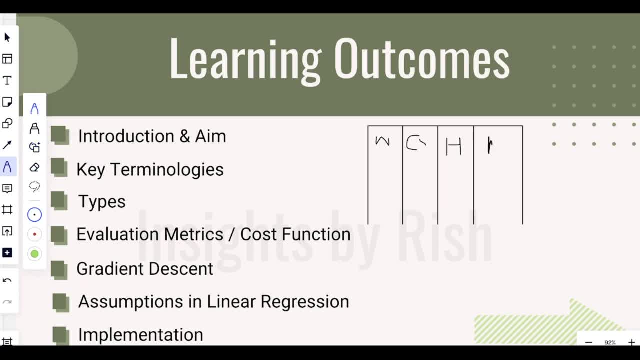 have to predict whether it will rain tomorrow or not. now the answer for this will be either yes or no, that either it will rain tomorrow or it won't. so the output of this is categorical: either yes or no, and nothing apart from that. this is a kind of classification task. it can be either. 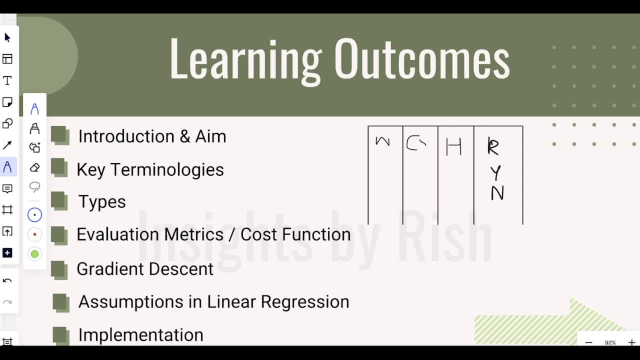 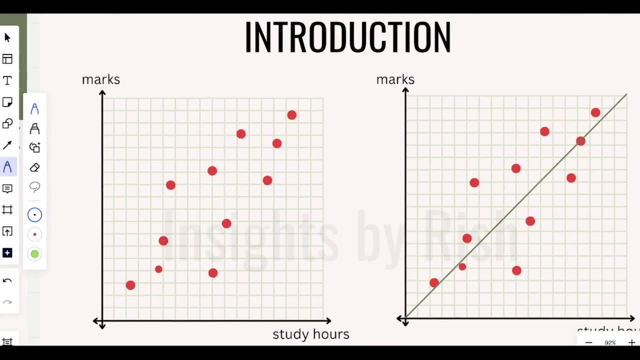 yes, no, true, false, 1, 0. and then can be multi-class classification as well, where you have more than what are two categories. so in this video we will be studying about a linear regression where our outcome will have continuous values. so, beginning with, in linear regression, we consider that there is a linear 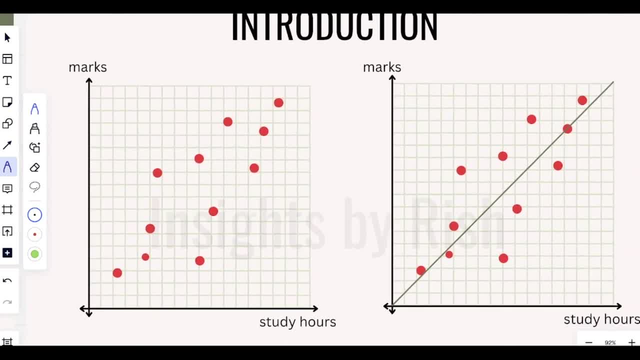 relationship between the x-axis and y-axis, between our X variable and Y variable, between this is our X and consider: this is our Y. now, this X is an independent variable. this X is an independent variable, which means it is not dependent on the variable, which means it is dependent on the variable. 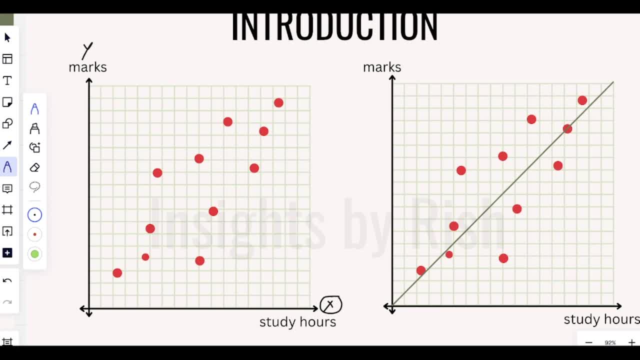 which means it is dependent on any feature. X is independent: it is what is given to us, so it is an independent one. well, Y is a dependent variable, which means it depends upon the input features. it will change as per the input features. so Y is a dependent variable and X is an independent variable, and in linear. 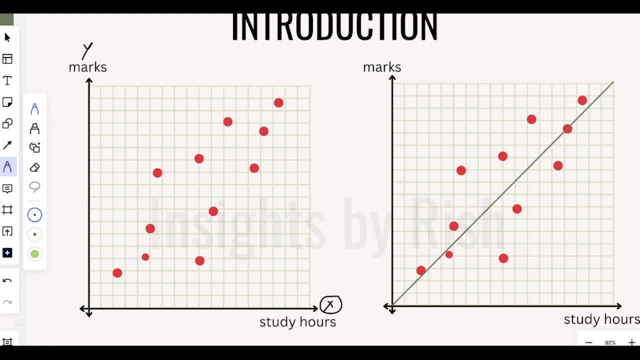 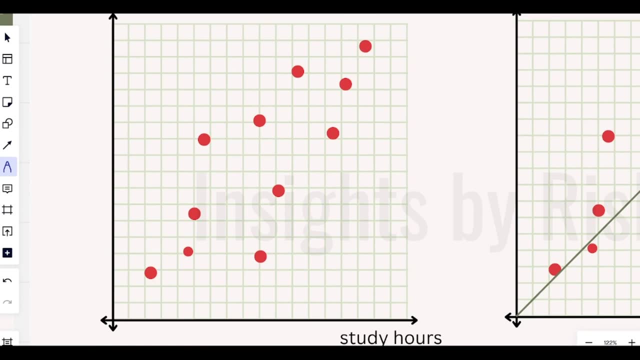 regression, we assume that there is a linear relationship between this independent variable and dependent variable. linear relationship means as the value on X increases, the value on Y also increases. so let us consider this. let's say for this point, for this point, this is the value an X. 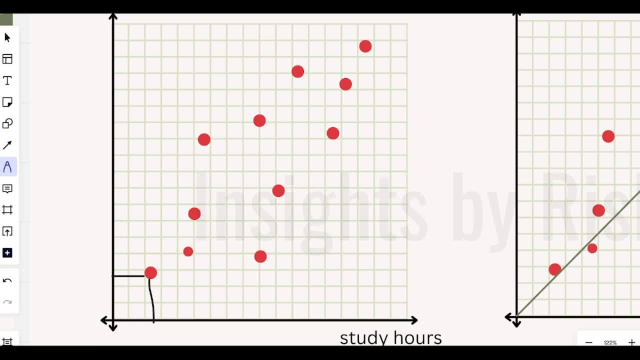 well, this is a value on Y. as the value on X increases. for this point, the value on X increases- let's say this was to, so this might have become full- as the value on X is increasing, the value and y also increases, let's say this also. this also increased, so for same for this variable, the value. 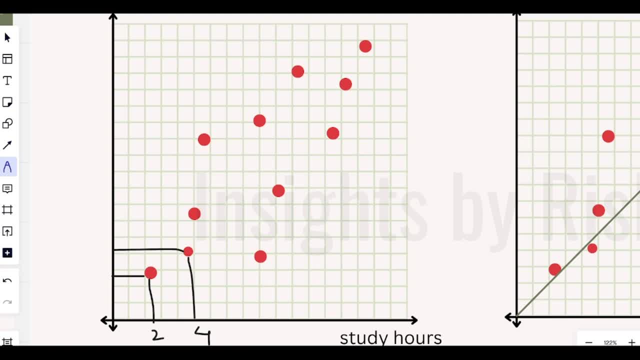 on X increase the value and y also increase, so this is a linear relationship. of course, we have some variables where a this won't be applicable. let's consider this one. for this, the value on x is increasing, but the value on y isn't increasing, so such kind of points are called as outliers where they differ from the. 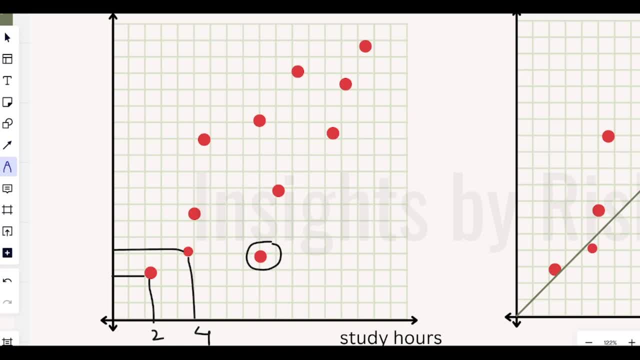 standard format where they do not follow the standardized techniques or standardized patterns. so such kind of data points are called as outliers, and we have outliers in all data sets available. so but maximum data points follow the linear relationship pattern, like if the value on x is increasing, the value on y is also increasing, and that's the basic foundation of linear. 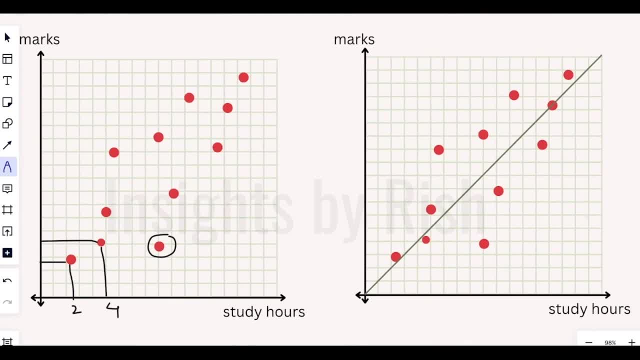 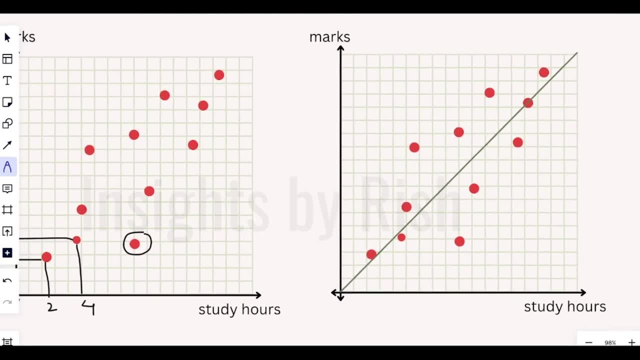 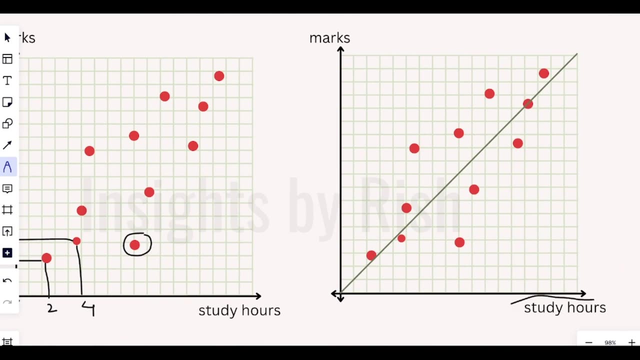 regression that we follow, that there is a linear relationship between our independent variable and dependent variable, for example. consider this example here: on x-axis we have study hours and on y-axis we have marks. now as the study hours increases, as we start studying for more and more. 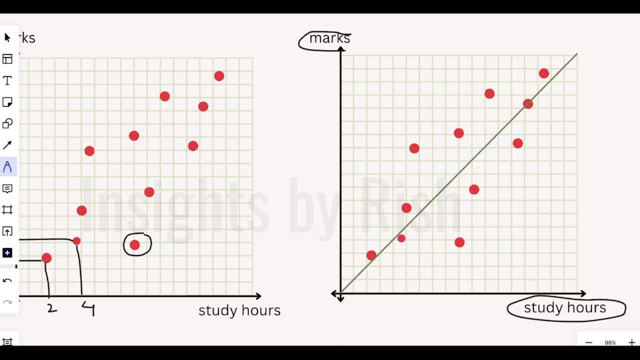 hours, the mark also increases. so this is a dependent variable and this is the independent variable. as your independent variable, that is, the number of hours you study- is increasing, your marks- that is, your dependent variable- is also increasing. that is, your marks are directly dependent on your study hours. 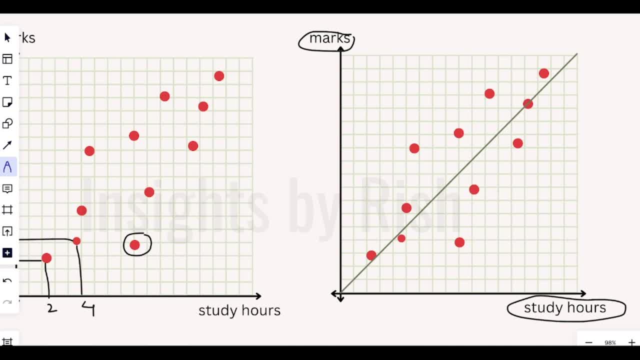 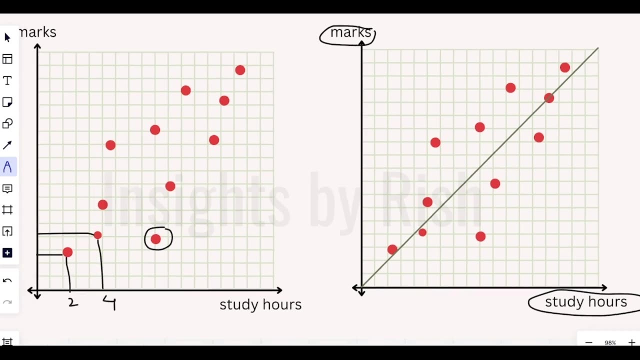 so this is the kind of linear regression where there is a linear relationship. when one variable, when one input variable is increasing, the dependent variable is also increasing. so the main thing that we do in this linear regression is to draw this line. this is a line initially. when we plot the lines, we have to draw the line that passes as close as possible from. 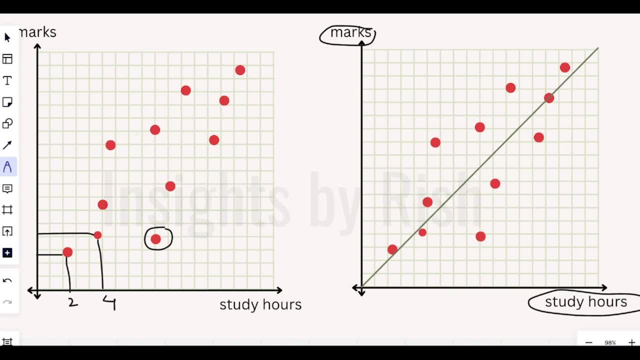 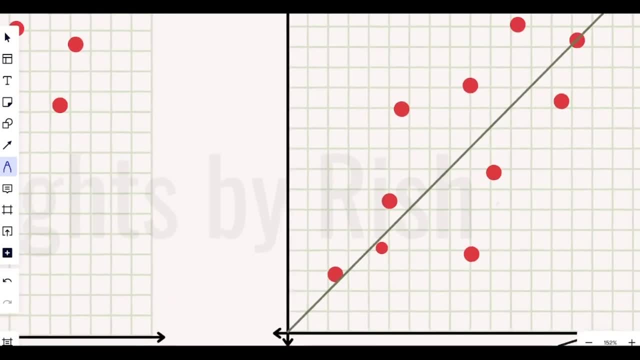 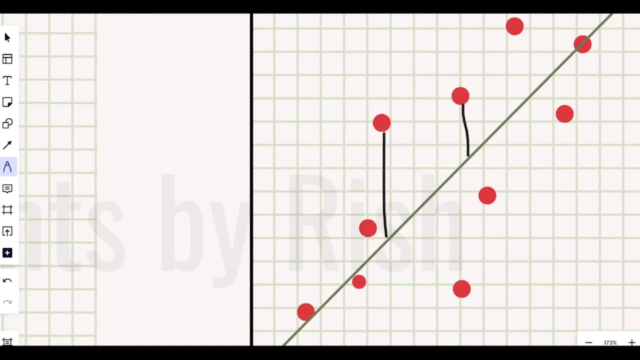 all these points. of course, we don't have the perfect data that that this line cannot pass through all the data points. what we have to do, we have to draw such a line that will have minimum distance from all these points. this distance from this point to this line should be minimum. 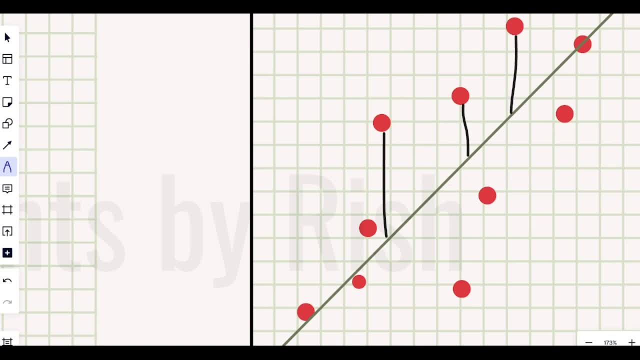 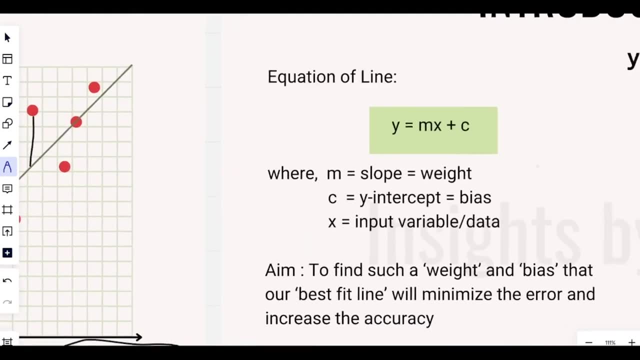 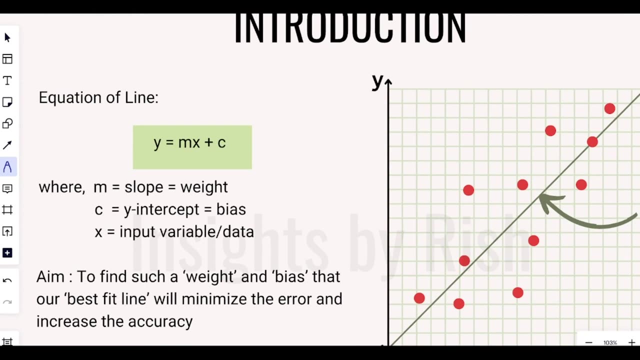 so we need to draw such a line that the distance between this point to this line is minimum applicable to all the data points. so moving forward, here we can. as we can see, the equation of this line is: y is equal to mx plus c, which is a basic mathematical equation. now the m stands for slope and c stands for y intercept. 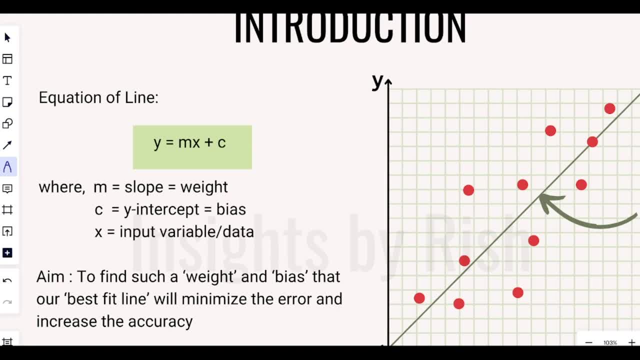 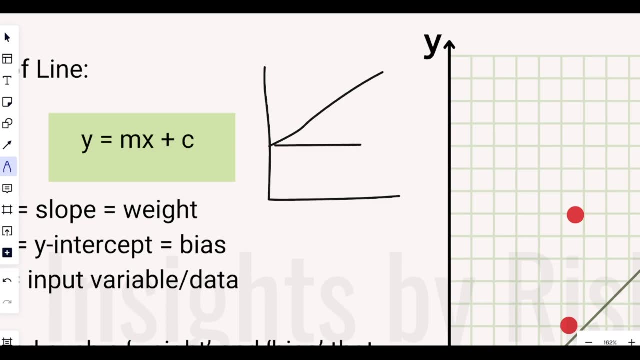 in machine learning we consider our slope as weight and our y intercept as bias. so let us consider: this is a graph and this is our line. so the angle angle it is making is a slope. the angle it is making here is your slope m, while the distance from origin up to that line is our y. 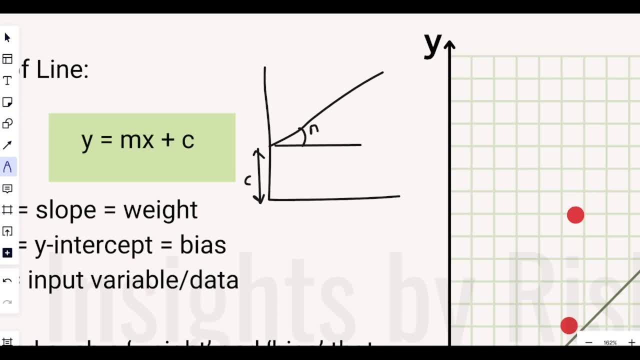 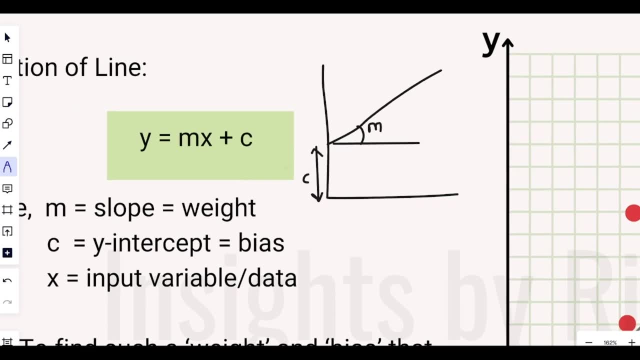 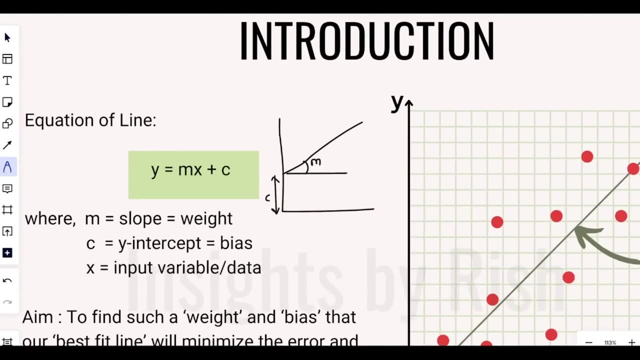 intercept c and this is your m. so this m is a slope, that is the angle it is making, and c is the y intercept in machine learning. m is weight and c is bias. well, x is your input variable. now, as you know, as we can, as we change this m and c, the line will also change. 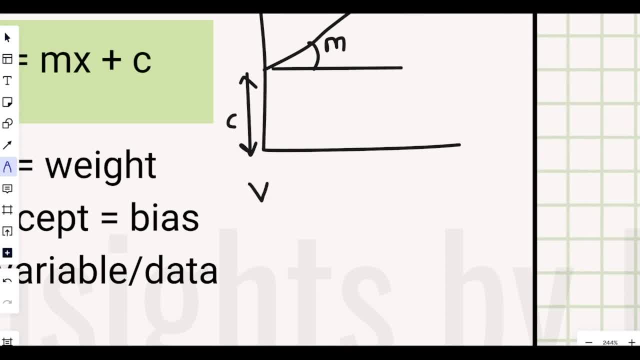 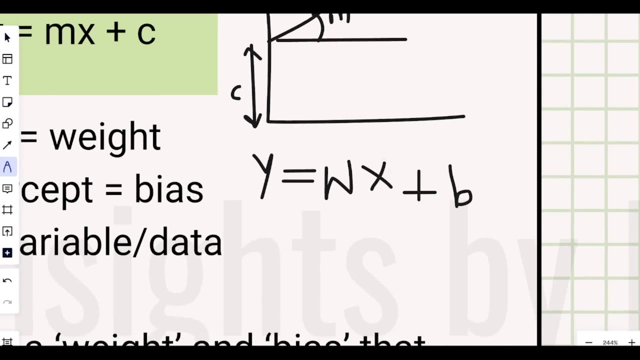 so if we write this equation in the input variable, we can write that y equals to. that's a expressing equation. if you write it in the terms of weight and bias, your y will equal to w x plus. so in this terms you can see x is a fixed value, x is a input value which is fixed, so you 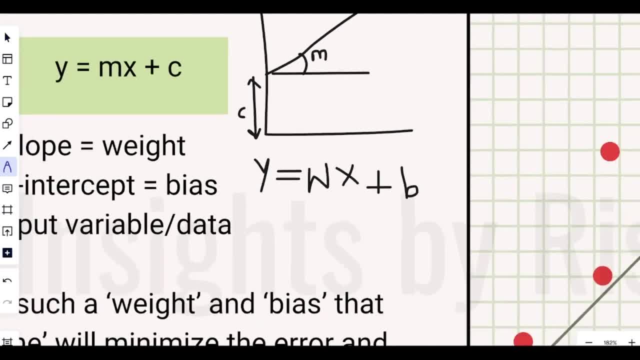 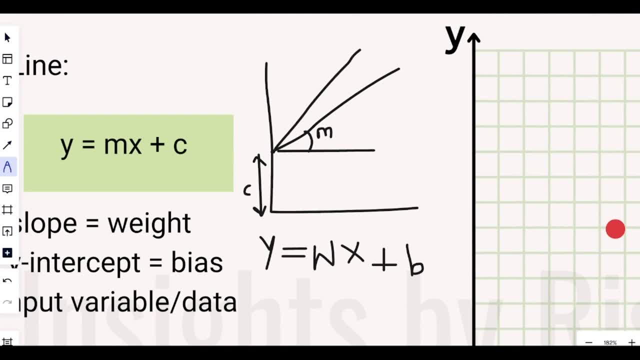 cannot change this. what you can change is your weight and b. so as you change your weight and b, the line will change. I've increased the slope here. If I increase the slope more, it will increase more. If I change the y-intercept, the line can start from here. So as I'm changing, 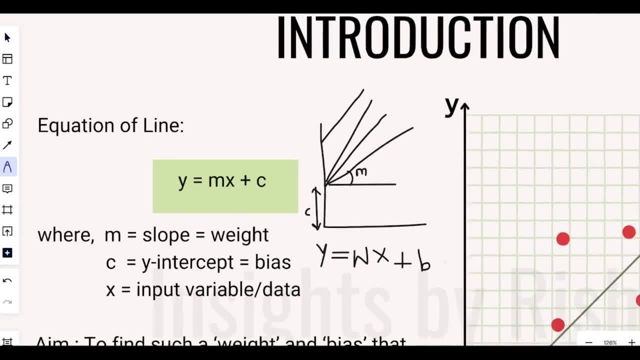 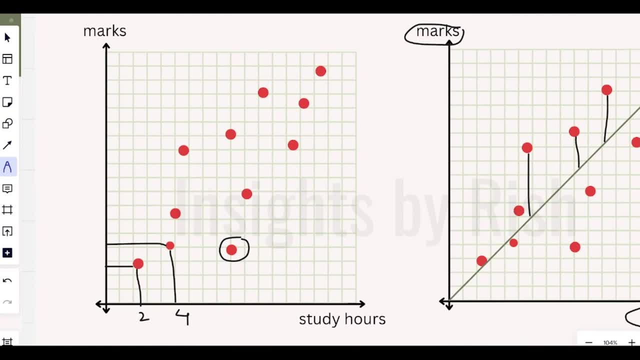 these features w and b, the line is also changing. So when I say that we have to draw a line that passes as close as possible from all of these points, there can be multiple lines. This can be a line, this can be a line and this can be a line. So which line to? 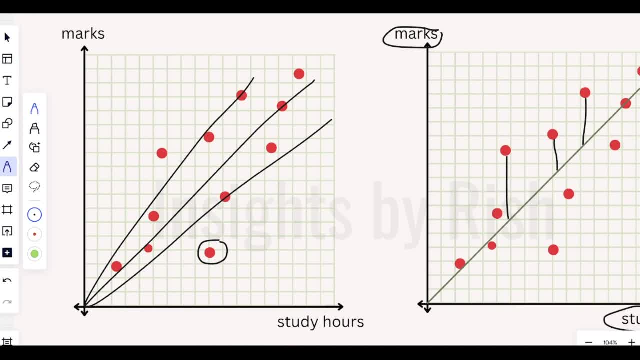 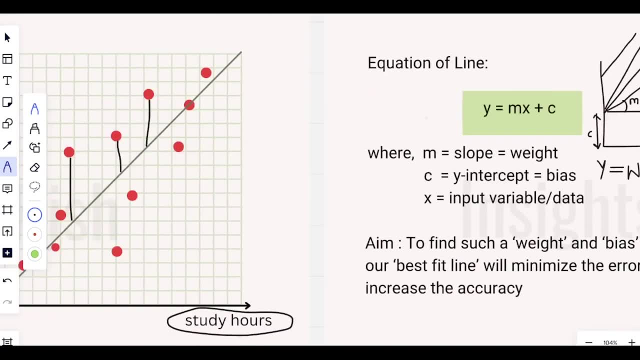 choose. There can be multiple lines, So this line changes depending upon the values of weights and bias. As the values of weight and bias- that is, this m and c- changes, the line also changes. So which line to choose Depends upon the distance between the points. 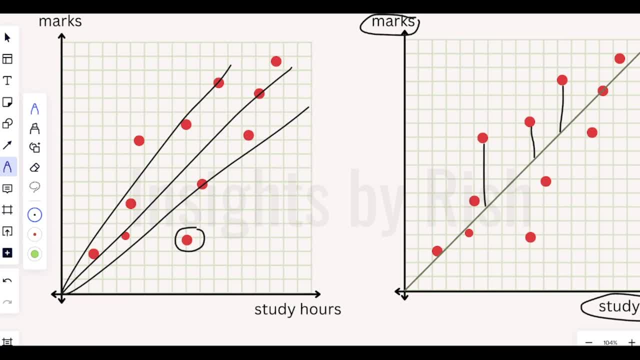 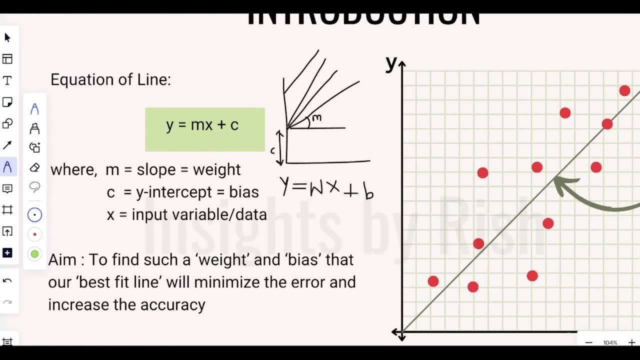 and the line. You have to choose a line that has minimum distance from this point to line, And that's how we compute error as well, which we'll study later in this video. So that's the basic understanding. Now we know that, as we are changing the weight and bias, this: 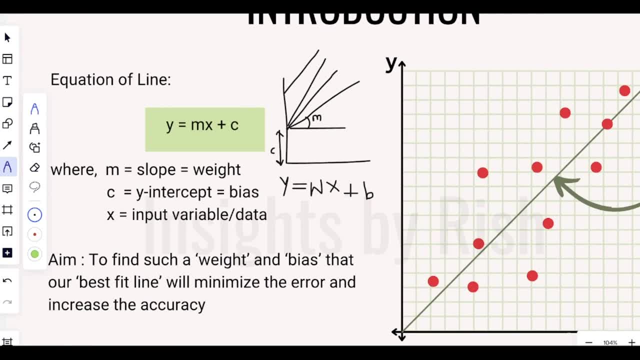 line is changing and we have to find such a line that is having a minimum distance from all of these points. So the main aim of our linear regression is to find such a weight and bias that our best fit line- this line is called as best fit line. We'll understand. 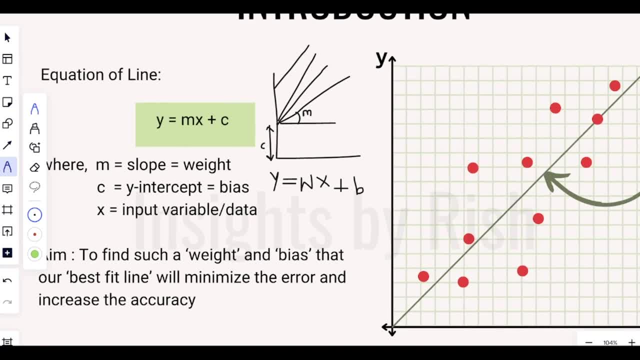 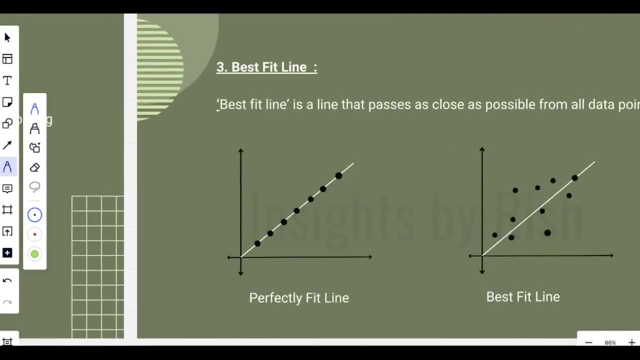 what it means. So to find such a weight and bias that our best fit line will minimize the error and increase the accuracy. What do you mean by best fit line? See, in this case, you know the line is passing from all the data points, It is passing through all available data points. 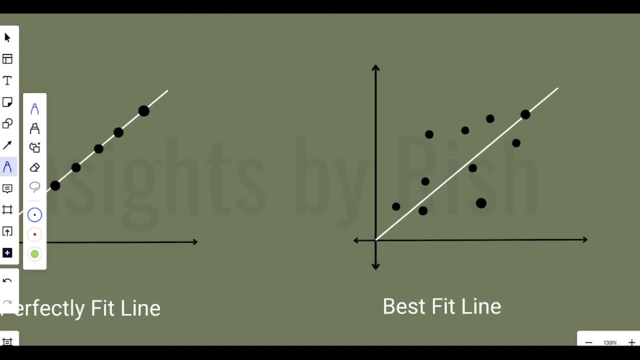 and such a line is called as perfectly fit line. Well, in this case, where the data, the line cannot pass through all the data points, but it at least tries to pass as close as possible from all the data points, and such a line is called as best fit line. When you 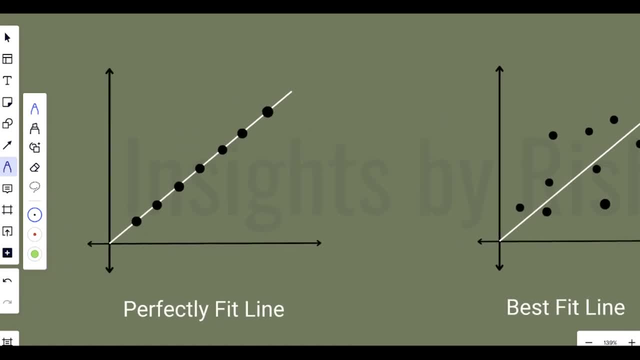 have perfectly linear data, that perfectly linear relationship. when you have between your x-axis and y-axis, the data is in this format. But you rarely get such kind of data in real-time environment where you have a perfectly fit line Most of the time you have. 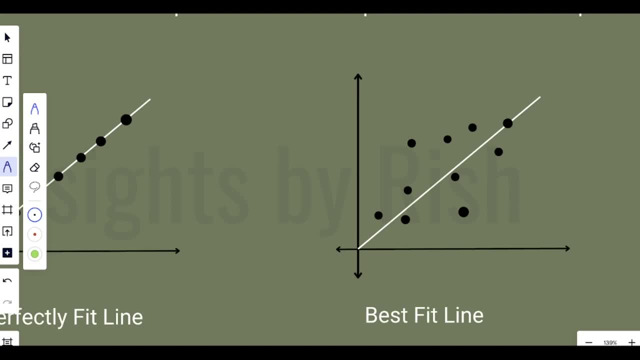 such data, though it is in a linear fashion, but it is scattered somewhere here and there. So the line that cannot pass exactly from all data points, but it tries to pass at least as close as possible from all the available data points, is called as best fit line. So here. this lines not pass through all data points, but it tries to pass at least as close as possible from all the available data points, is called as best fit line. So here we will tell you the basic knowledge First. what we do know is this, which we know well, we will not. 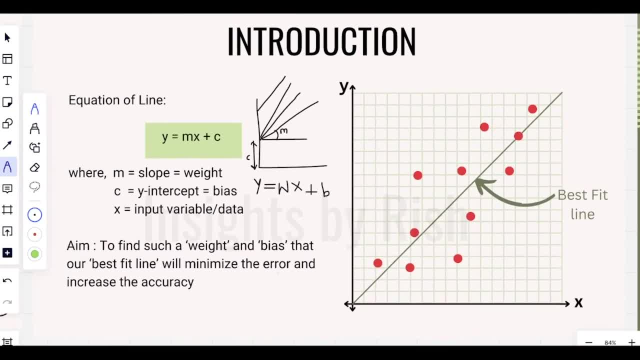 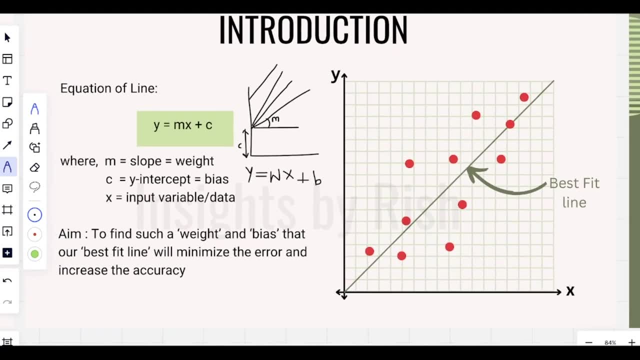 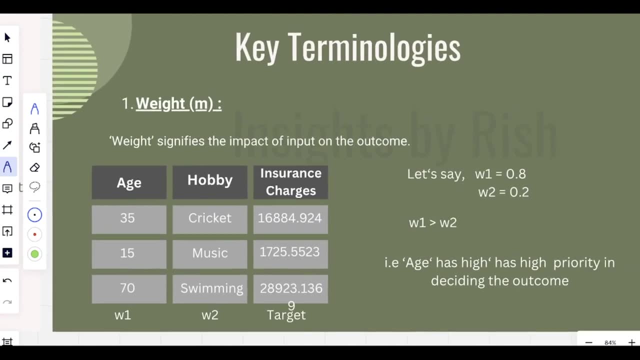 our main aim is to find such a value of weight and bias that it that it will plot a best-fit line which will have the minimum distance from all of these points. now, what's the significance of this beta and bias? understanding that, firstly, weight. now weight signifies the impact of input on our outcome. see when. 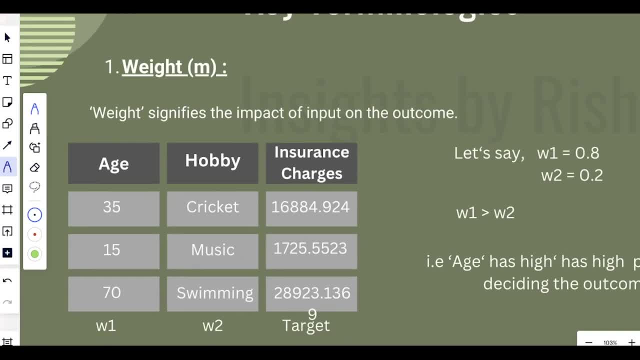 when you have multiple input features, your output it depends on the input features, but every input will have different impact on your output. let's consider this example. in this example, you have to predict the insurance charges depending upon the age and hobby of a person. so here you have two. 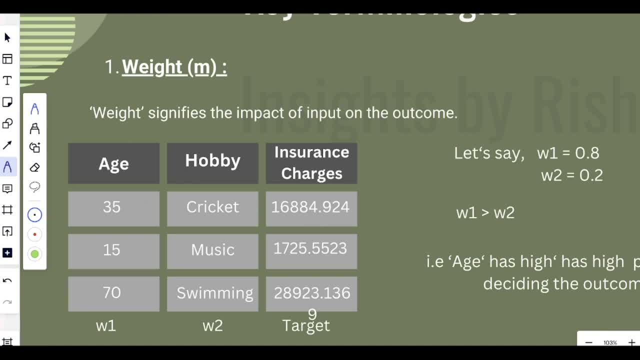 features- age and hobby- and depending upon which you have to predict this insurance charges. now, every column, every feature, has a weight associated with it. let's say, w1 is the age associated with weight associated with age column, w2 is the weight associated with hobby column, and you have to predict this insurance. 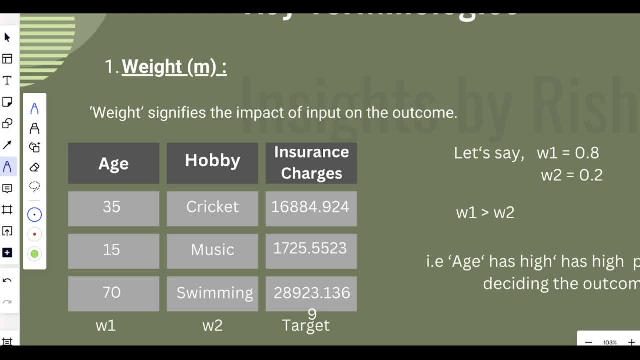 charge. now, age. age is an important factor in determining the insurance charge, like. but the hobby isn't an important factor like. you cannot ask, you cannot predict the charge insurance charge depending upon a person's hobby. so the age is an important factor in deciding the charge. well, hobby isn't. as a human we can. 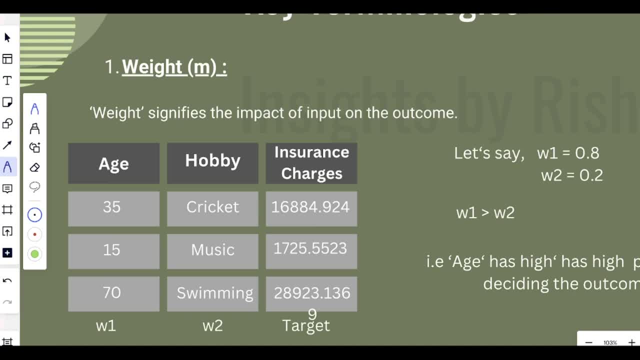 understand this pair observation, but for the machine we need to plot it in a numerical fashion. let's say, the weight associated with this age column w1 is 0.8, is 0.8, while the weight associated with this hobby column is 0.2. now here we can. 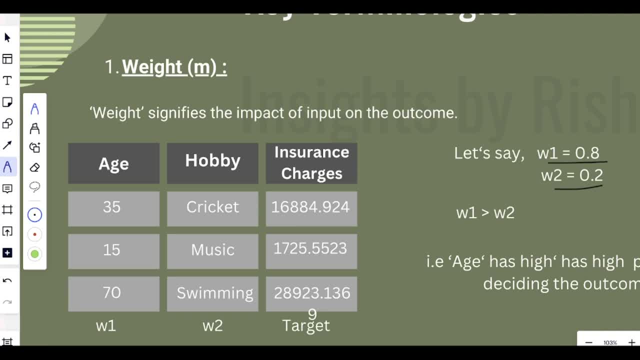 clearly see that the weight 1, which is the weight associated with age column, is greater than the weight associated with hobby column. so here we can say: we can conclude: from this observation we can conclude that the age column has higher impact on our target variable, that is, on our outcome insurance charge, rather than 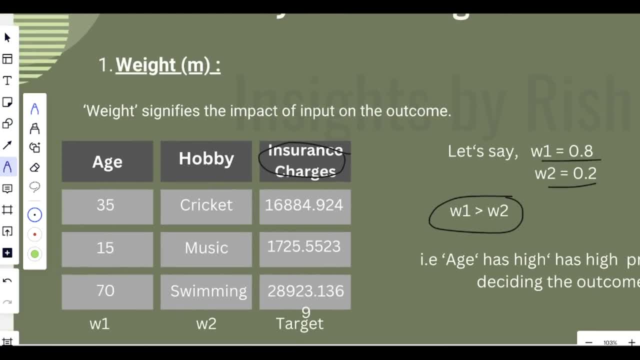 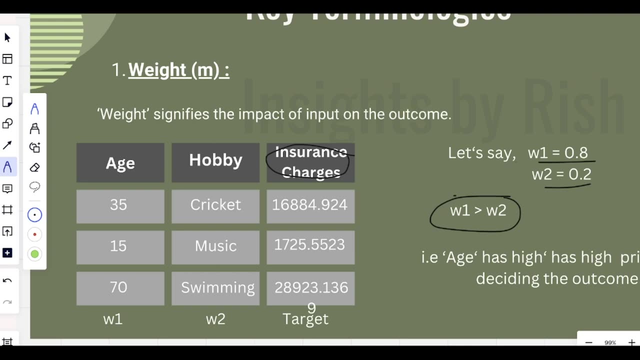 hobby. so the input feature that has higher weight has high impact on target variable, while the input feature that has lower weight has less impact on our input feature. so that was in significance of weight where, which helps us to understand the impact of an input on the outcome, while the bias- now the bias again- has an 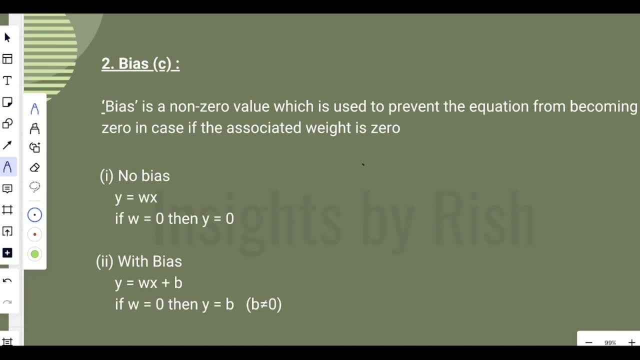 important role to play. let us consider that we have an equation without bias. let us consider equation without bias we you have: Y is equal to W, X, and we are assuming that we don't have any bias. now this weights and bias are initialized by our model, our machine, our library, scikit-learn. so let us consider that. if 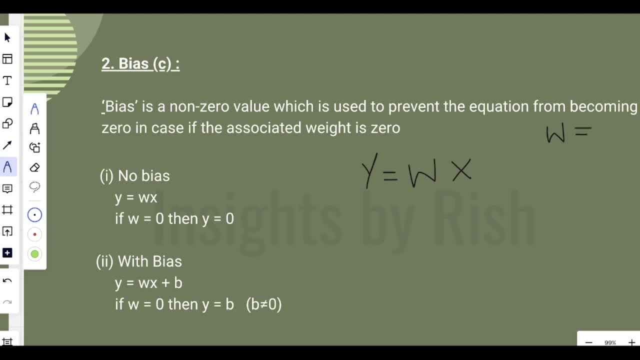 in case the weight is initialized to 0. if our model initialize the weight to be 0, in that case the whole element will become 0, because anything multiplied by 0 is 0. so in in such case- though it is a rare case, but it can happen- that if the 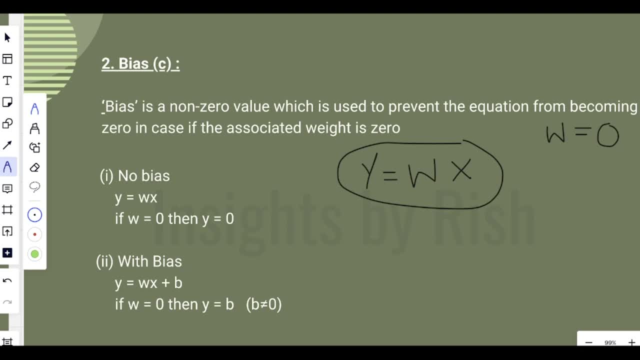 weight is initialized to 0. in such case, your whole element will tend to 0. to prevent this from happening, you add a nonzero term bias into it. now what will happen? though your weight is 0, but still your Y will won't become 0 because it has some nonzero value B. so to prevent the element from turning to 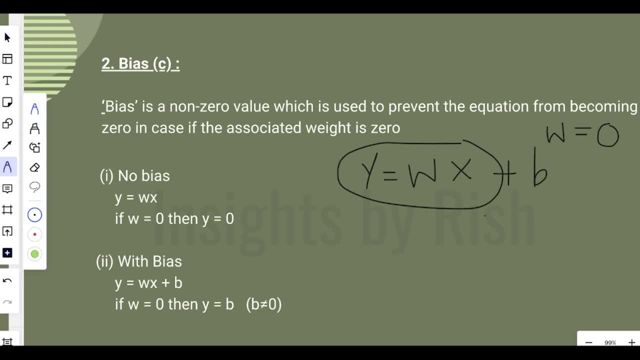 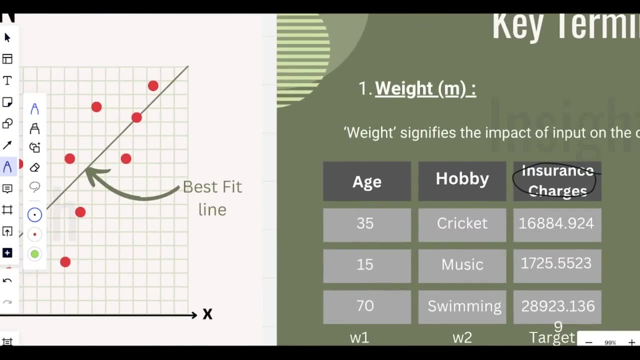 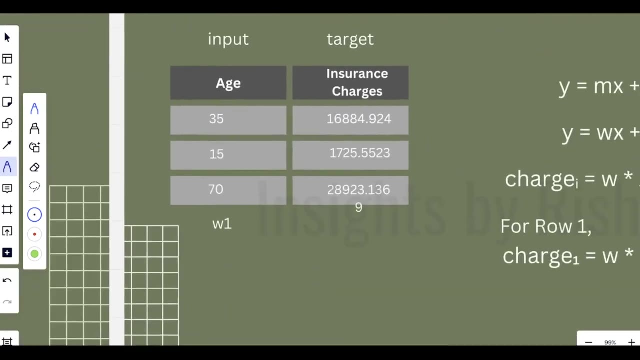 0, you add bias, so bias is an important factor that prevents your element from turning to 0. now that we have understood all the key terminologies, we'll move ahead to the types of linear regression. so we have two types of linear regression, like we have. 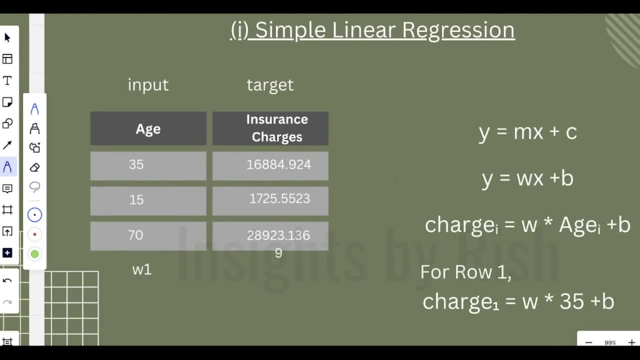 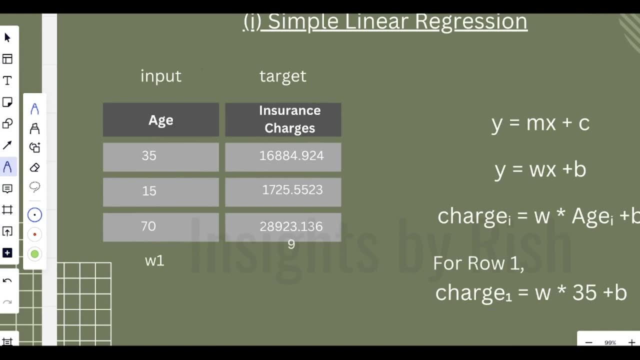 many types of linear regression, but the most popular one are simple linear regression and multiple linear regression. so in simple linear regression we have only one input feature and our outcome- that is, our target variable- is dependent on a single input feature. now here you can say: we are predicting. 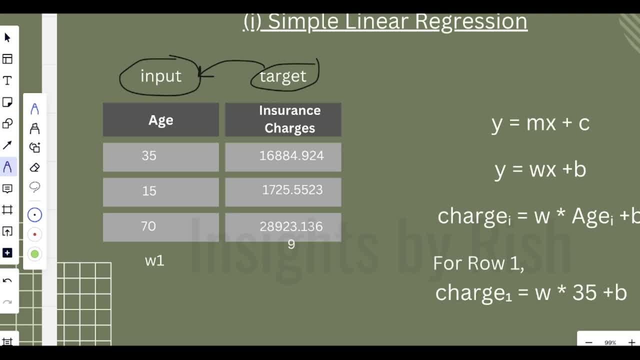 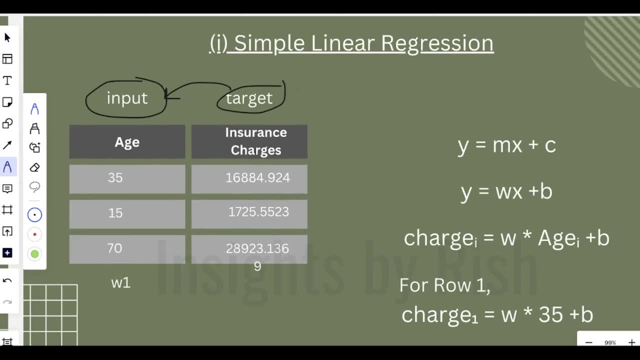 the insurance charge depending only upon H. we can input the H and the model will predict the insurance charge. so in simple linear regression we have only one input feature and we are predicting the depending upon only that single input feature. in that case we have a simple line equation which is: Y is equal to W, X plus B. 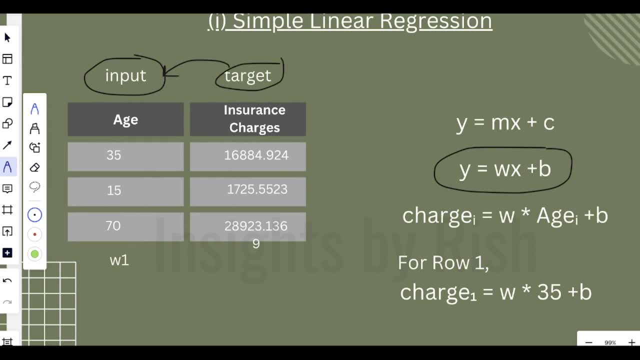 where your Y is your insurance charge at I which you are going to predict, W and B are the terms that your model, your library, will generate depending upon the iterations and trial and error, and X is the input age: age at I. now, if you consider row 1, if you consider this row 1, 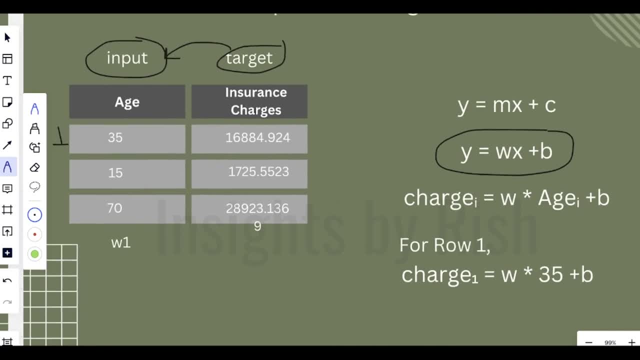 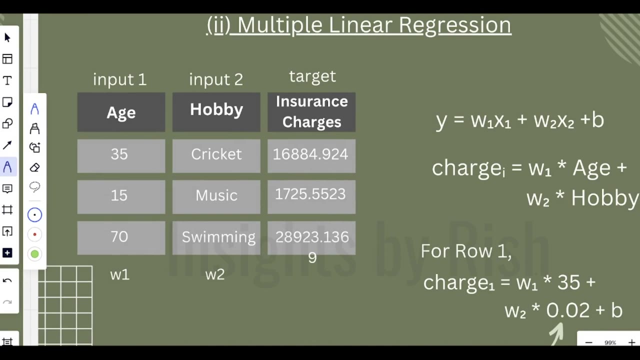 here the charge at 1 will be equal to weight into the input 1, that is 35 plus B. same for row 2 and row 3. now in multiple linear regression you can have multiple input features like in simple linear regression. we have just a single. 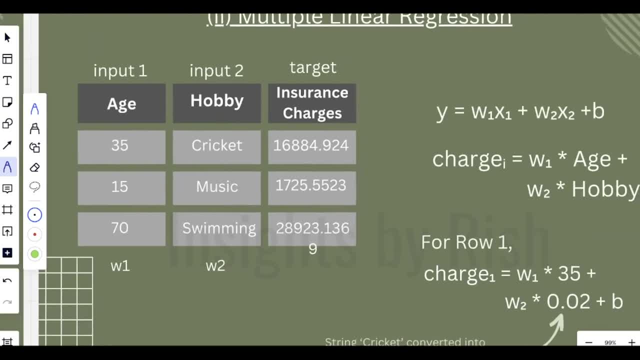 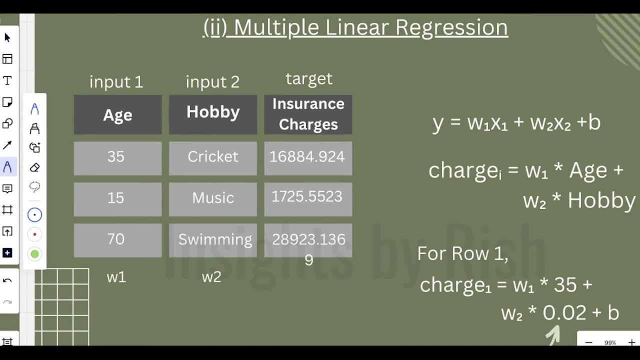 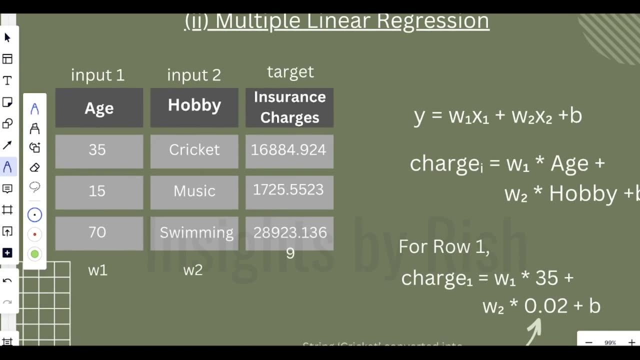 input feature, while in multiple linear regression you can have n number of input features and your target variable. your outcome will depend on that n input features. now, for example, here I have considered two input features- age and hobby- and I am predicting insurance charge based upon this two input features. so in this, 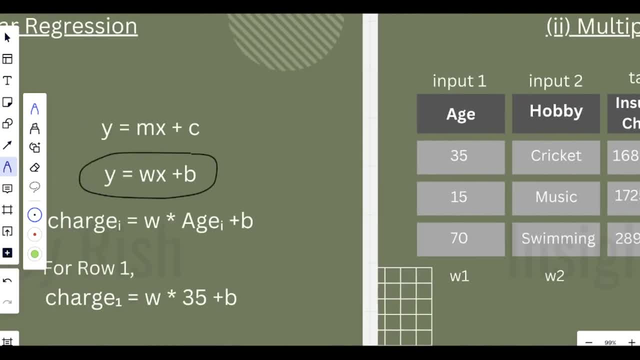 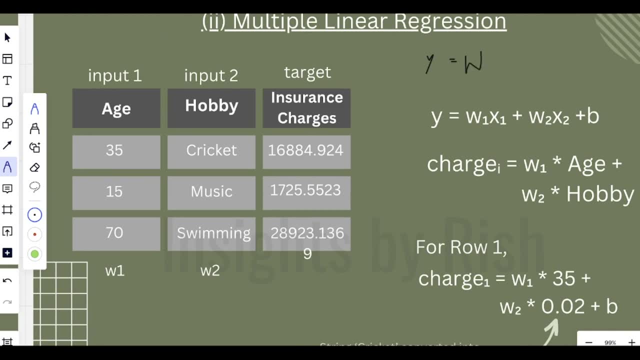 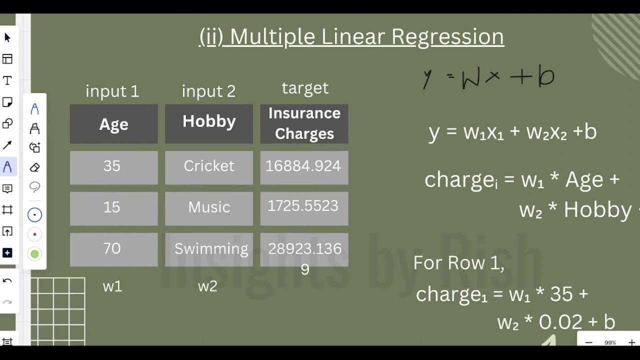 case the simple line equation is extended, like the normal equation that we had was Y is equal to W, into X plus B. this was a simple line equation that we had in a simple linear regression. now in multiple linear regression we in, we expand it to n number of points. let's say for point 1, that is, for input 1, it. 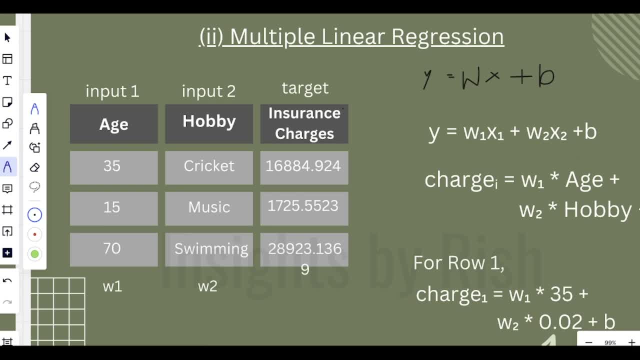 will be W and X 1. for input 2 it will be W 2, X 2, like this. up to nth point it will be W and X n and plus biased term. in this case you can see the W 1, W 2 and B. 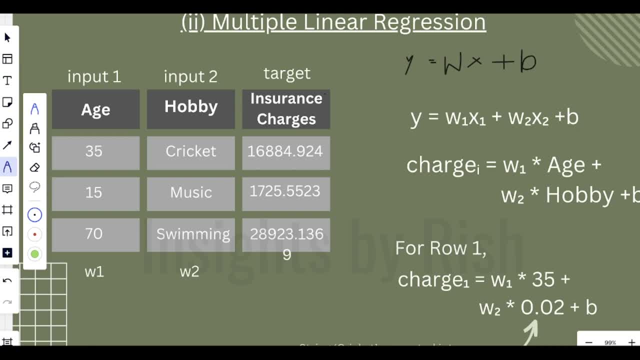 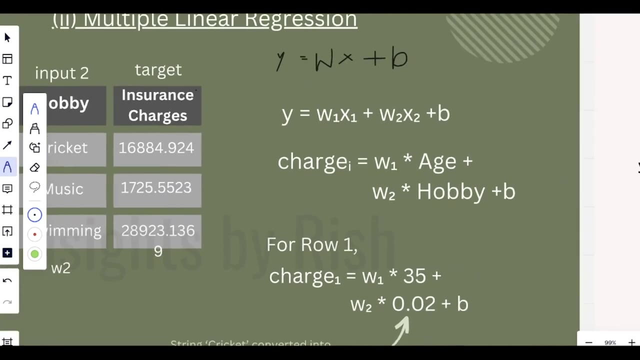 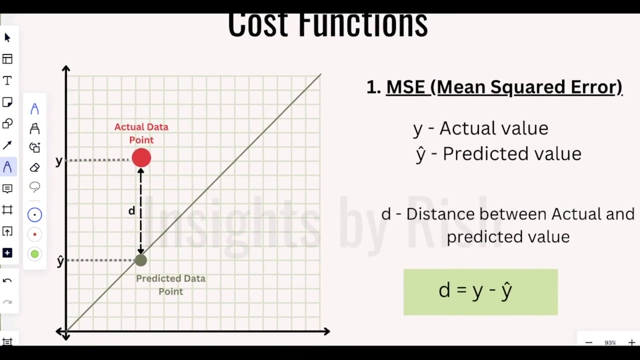 are all these factors that will be generated by our library or generated by our model itself, depending upon the trial and error and iterations. that's the basic difference between simple linear regression and multiple linear regression. now moving forward, let us understand the cost functions. cost functions are basically used to evaluate your model. you have to see how much. 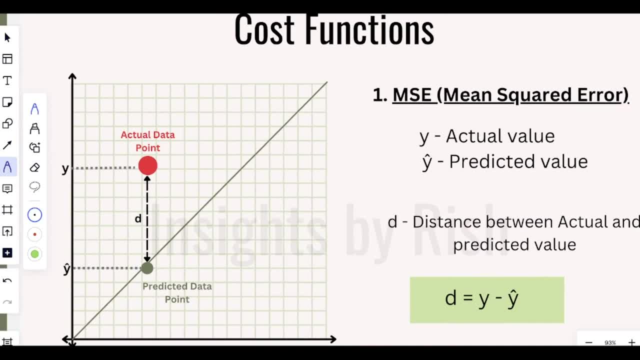 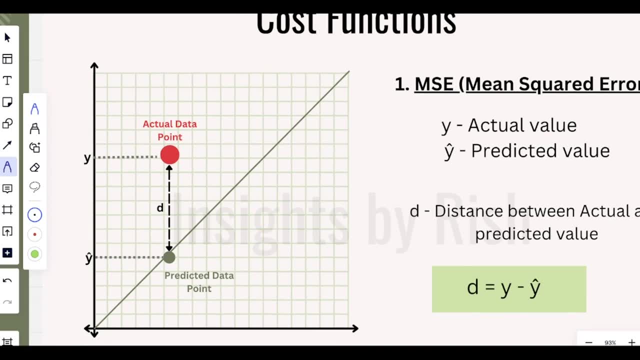 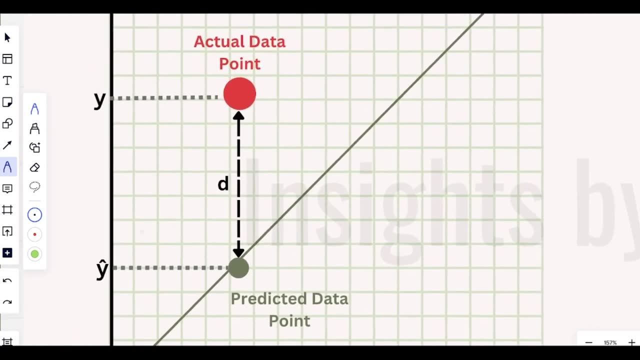 error your model is reporting and how much accurate your model is. there are multiple types of cost functions that we have in linear regression. let's start with some basics first. you have this is your actual data point. for an example, I consider your only a single data point. this is the actual data point. you will map that data point onto a best 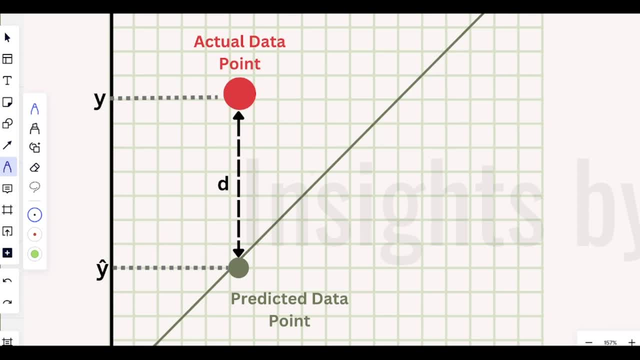 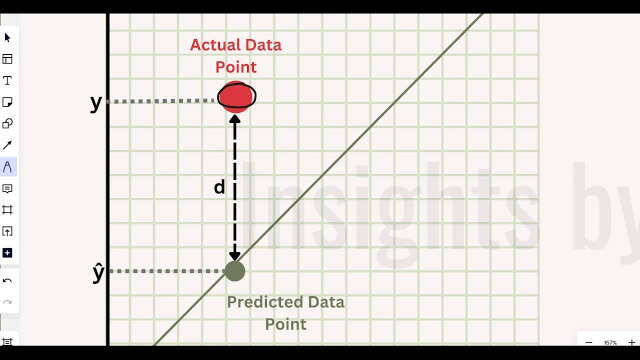 fit line. this best fit line is also called as regression line. they will map that your actual data point on your regression line. this is our actual data point, which is symbolized with Y, and this is our predicted data point, which is symbolized with Y. hat, the actual data point is symbolized with Y. and when you 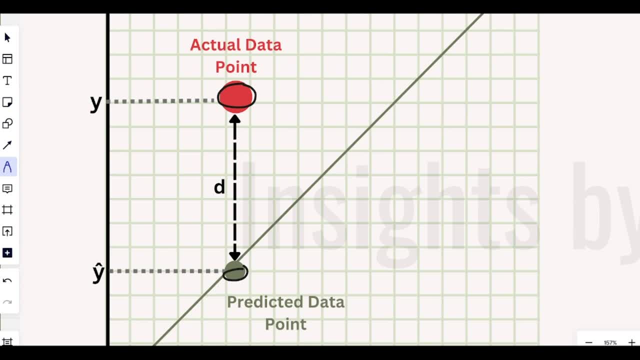 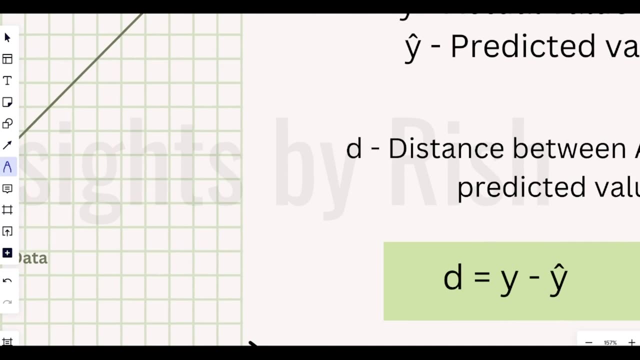 map that data point onto this regression line. it is symbolized with y, hat and the distance between both of them is symbolized with d. now, when you have to find this d, d is the difference of actual data point and predicted data point. so the formula for d is this actual data point, which is y. 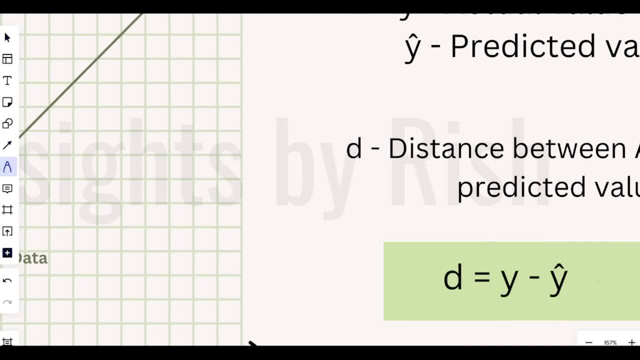 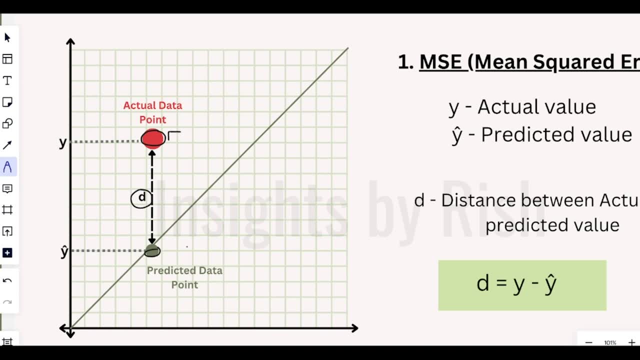 minus predicted data point, which is y, hat and d is the difference between both of them. let's say that you, actually the value of your data point, is 5 and the model has predicted it to be 3, then your distance, your d, will be 2, that is, 5 minus 3, 2.. so the first cost function that we 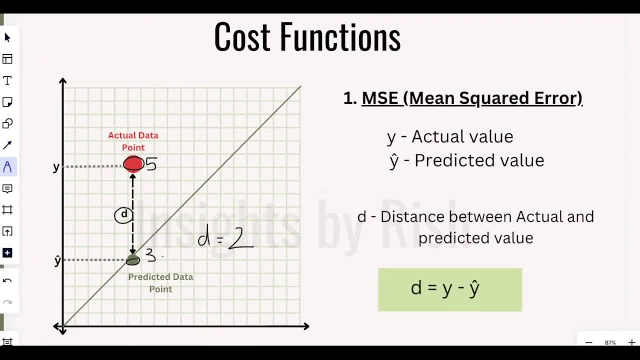 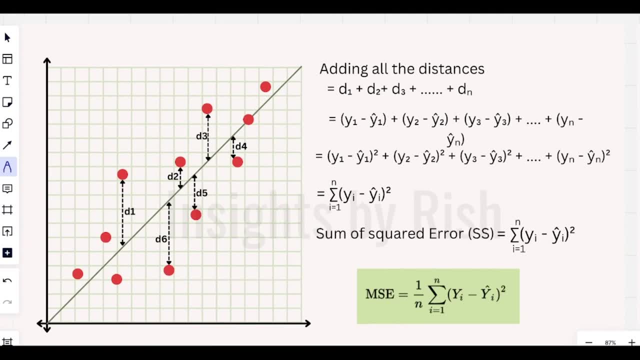 have in linear regression is mean squared error, mse. so, as in the previous slide, we took the difference of only single data point for an example. similarly, you have multiple data points and you have to take the difference between them of every data point. you have to take the distance from first data point. 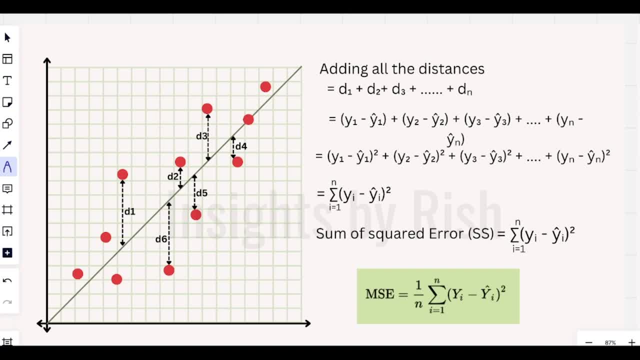 to the regression line. so you have to do this for all n data points. you have to take the difference between data point and the regression line for all the available data points. let's say D1 is the distance between the first data point on to its predicted one. D2 is the distance from the second data point on. 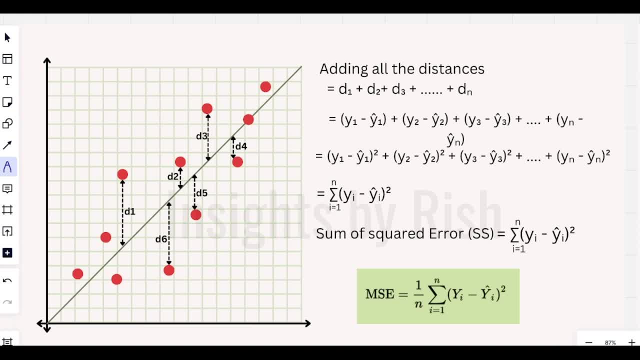 to its predicted one. so in such a way, you take the distance for all the data points and you add them up. so, starting with D1 up to Dn, you add all the distance starting from the first data point up to nth data point. now, as in a, 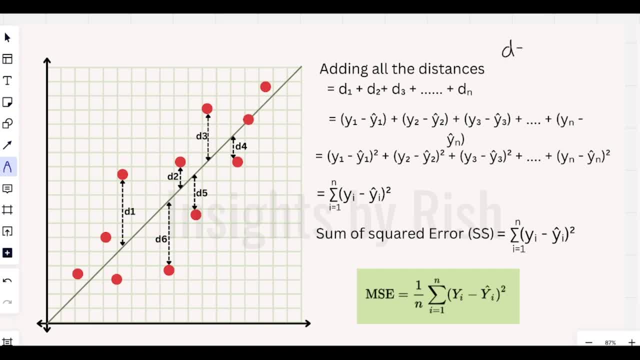 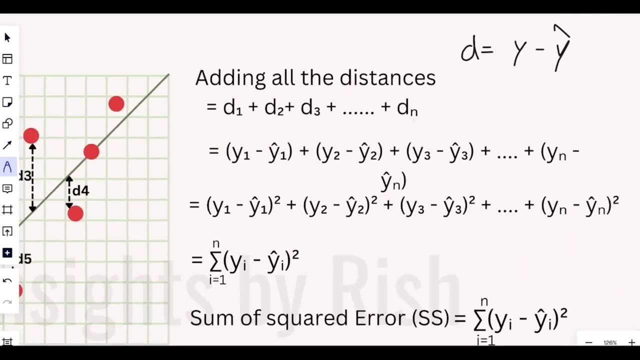 previous slide we study that a formula for D is the value of actual data point minus the value of your predicted data point, which is y hat. so this was for a single variable. now for we can expand this equation: for D1, we can write it as y1 minus y1 hat plus. for D2, we can write it as y2 minus y2. 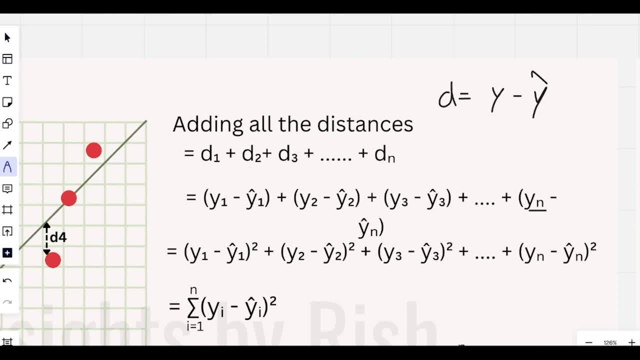 hat up to nth point is yn minus yn hat. now, in some case it can happen that the predicted value is greater than the actual value. let us consider that our model predicted a value to be 5 and let's say the actual value, actual value, this yth value is 2. in that case, your predicted 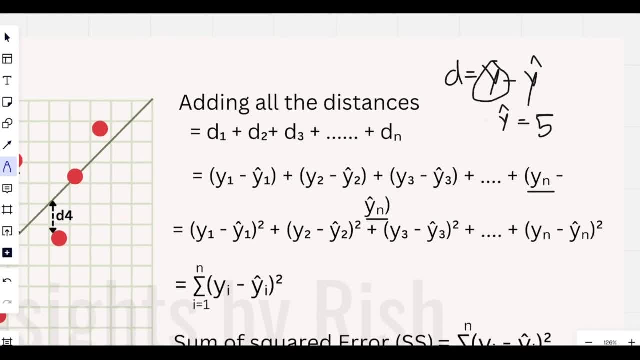 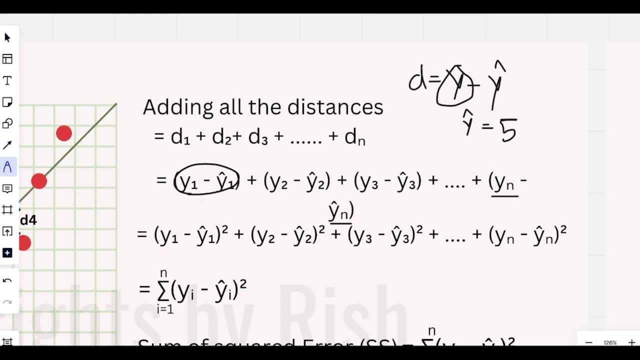 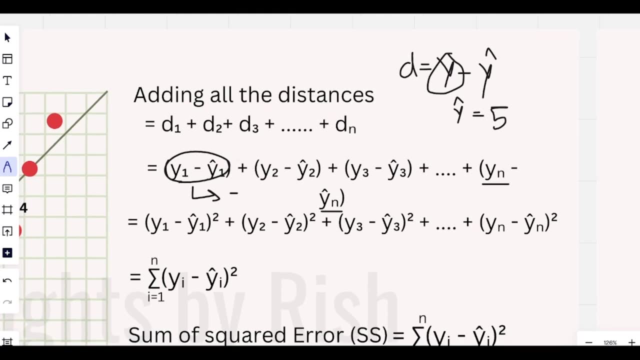 value is greater than your actual value, then in such cases it can happen that you may get a negative value now for this element. if the predicted value is greater than your actual value, then the answer you will get will be a negative value. so to prevent this negative, you square it up, you, you take. 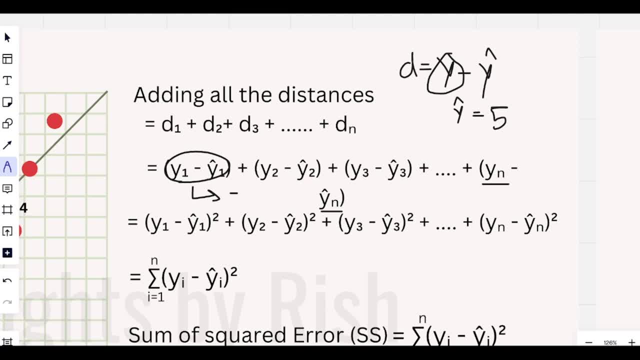 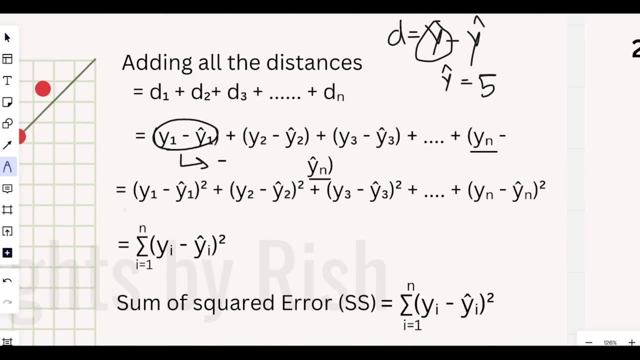 the square of y1 minus y1 hat up to nth data point. so you are squaring it up to prevent the negative data values. now we can generalize it. now this is this is our equation, and we will write it in a generalized form, which is this: 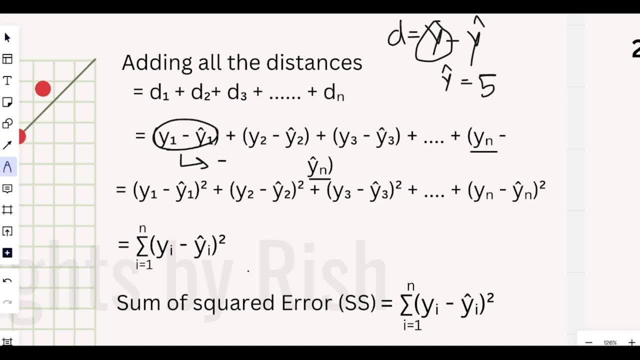 so summation of i is equal to 1 up to n. y i minus y. i hat square where i can start from 1 up to n. so summation of i is equal to 1 up to n. y i minus y. i hat square where i can start from 1 up to n. 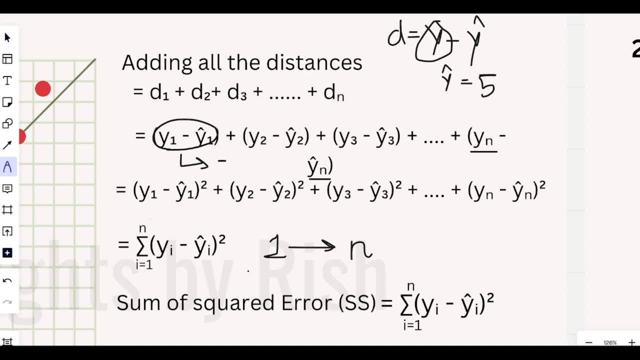 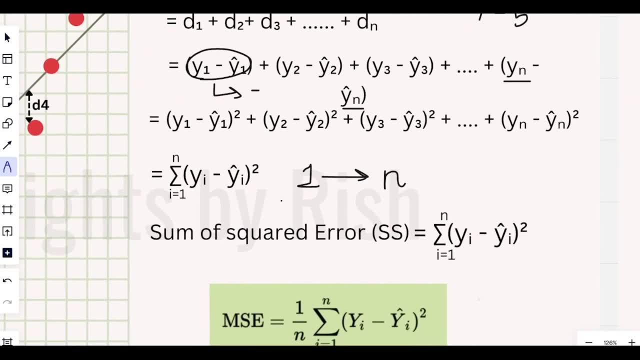 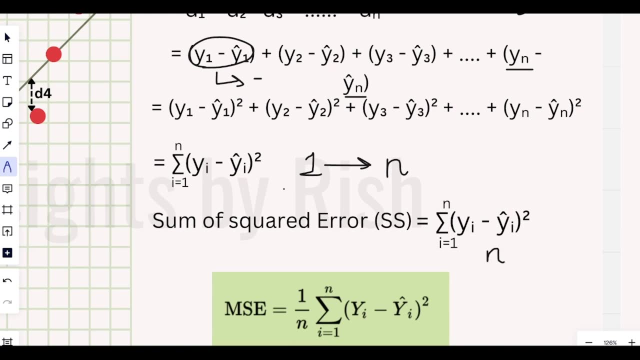 this is a generalized form and this generalized equation is called a sum of squared errors. this generalized equation is called a sum of squared errors and when you divide the sum of squared errors with total number of data point, that is n. let's say n is total number of data points that you have when you 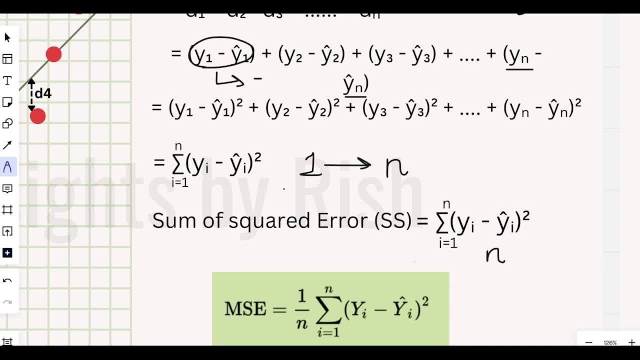 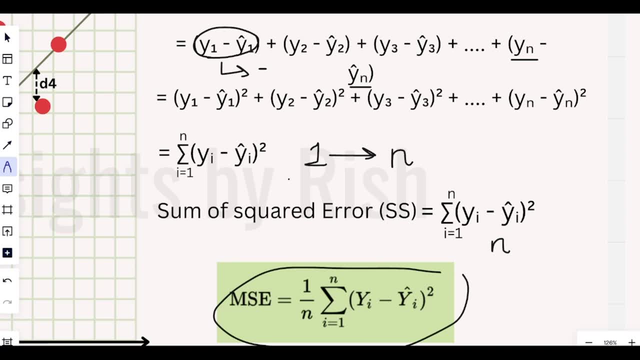 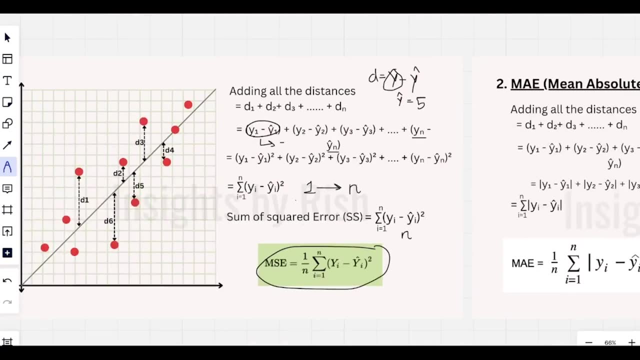 divide the whole sum of squared error with the total number of data points, you get mean squared error. this is your mean squared error. It is 1 by summation of i is equal to 1 to n. yi minus yi hat square. So this was the first cost function that we have, first evaluation metric mean squared error. 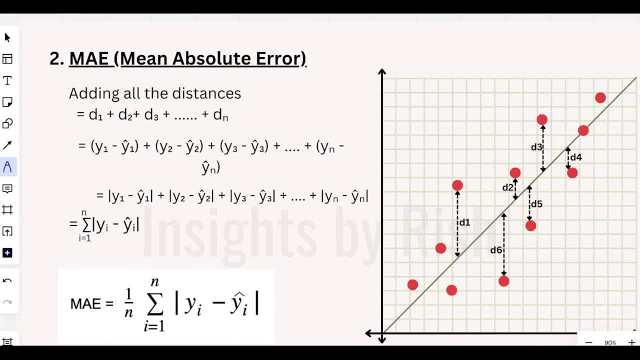 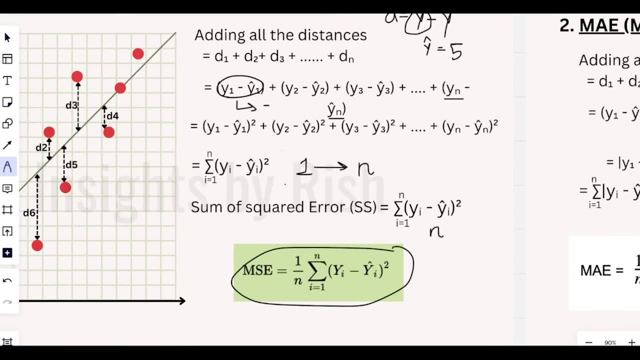 The second one is mean absolute error. Mean absolute error is very similar to mean squared error. The only difference is that in mean squared error, to prevent this negative values, to prevent this element tending to some negative value, we took the square of it. 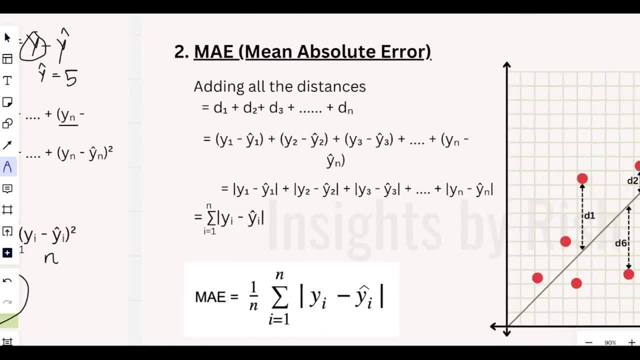 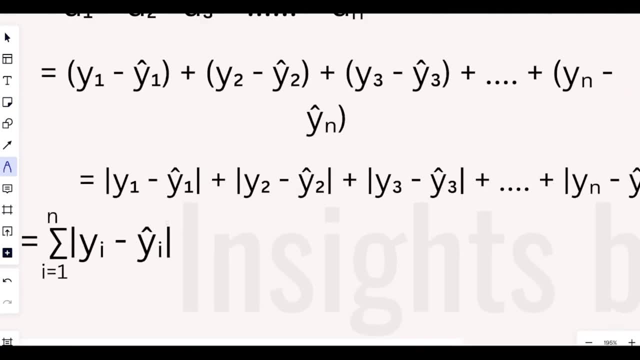 But in mean absolute error. what we are going to do is: you take the absolute, you take the modulus of that element In order to prevent the negative values instead of squaring it up. you take the absolute, you take the modulus of that element. absolute values. 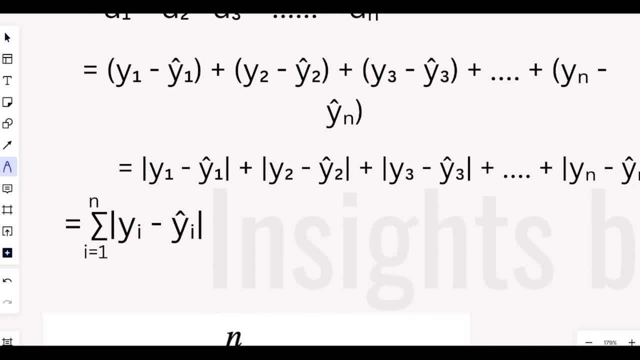 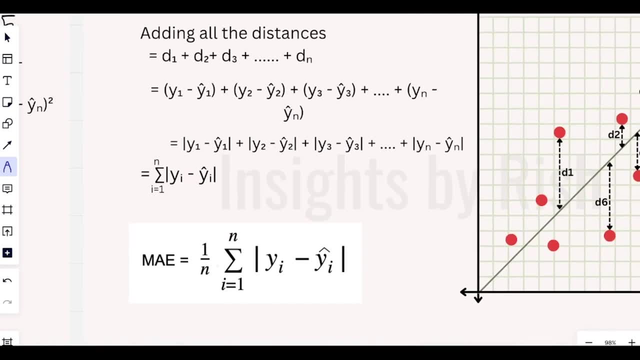 And then the whole equation is same up to nth element. Then you take a generalized form of it and you divide it, the whole, this equation, with total number of data points that is n, and you get your mean absolute error. So it is very similar to mean squared error. 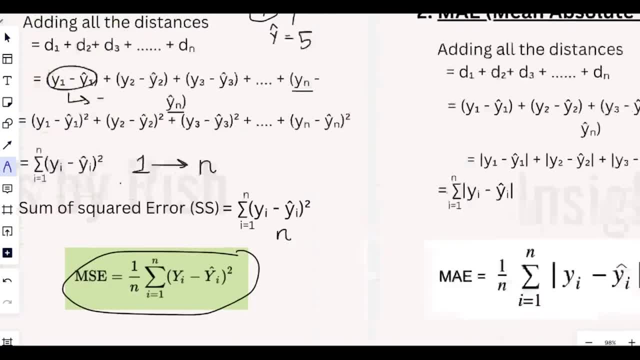 Only difference is that you take the absolute, you take the modulus of that element and you divide it. So the difference is: here you have modulus and there you have square. The third cost function is root mean squared error. In root mean squared error, you take the root of mean squared error. 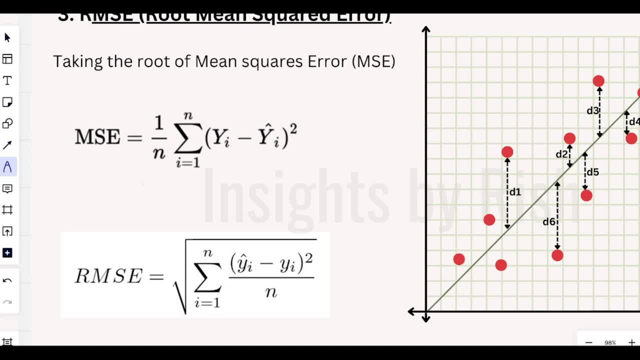 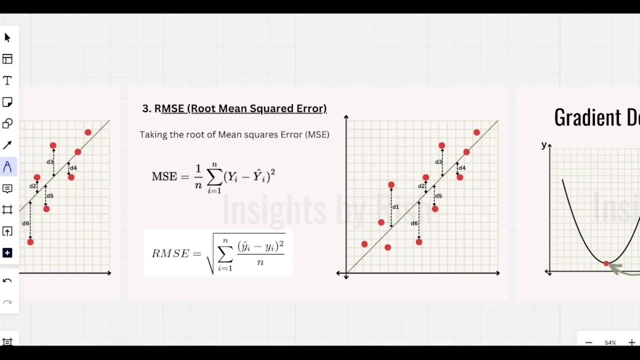 Now this is your mean squared error and you take when you take the root of it, it will be root mean squared error. So this was your third cost function. There are more. there is R2 score, adjusted R2 score, but we just studied the popular ones and most frequently used ones. 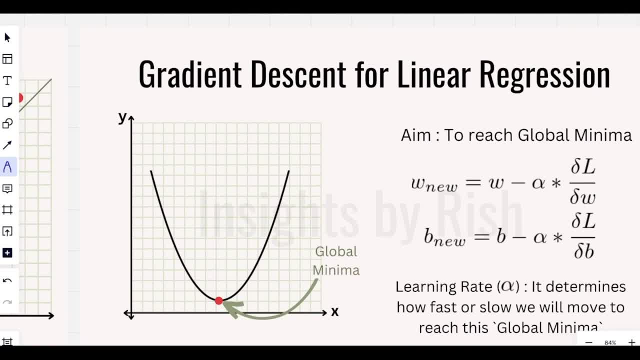 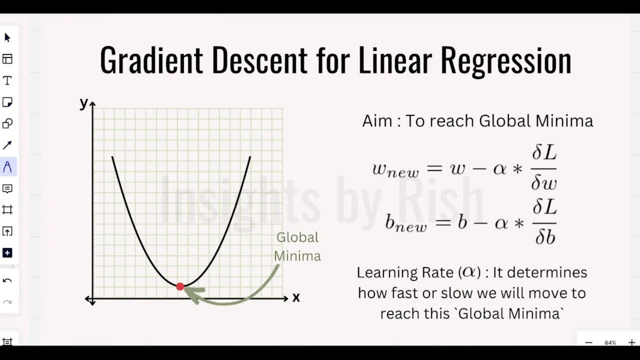 So, moving to an again an important topic, Which is gradient descent for linear regression. Now, what is gradient descent? Basically, this is the kind of parabola we have, And the gradient descent is an optimization strategy. Now, what is an optimization strategy? 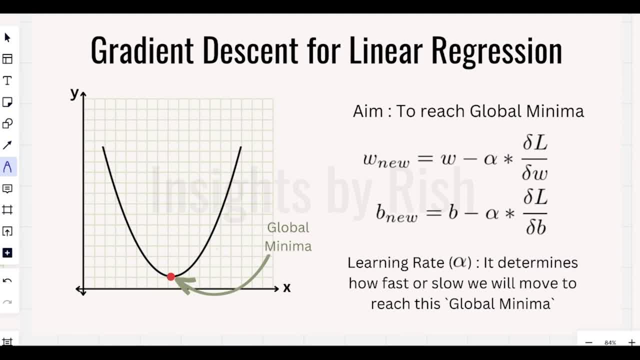 Here you know that we have to plot a best fit line such that it will minimize the distance from the data points. So this best fit line will change its position depending upon the weight and bias. So here we have to find the best fit line depending upon the weight and bias. 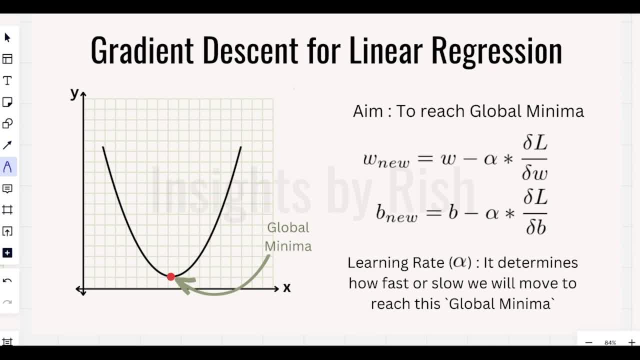 So, which means we are optimizing the values of weight and bias until and until we get the perfect, best fit line. So here we are optimizing the weights and biases, for which we require the understanding of gradient descent. Now let's say: first you have found, let's consider the mean squared error metric. 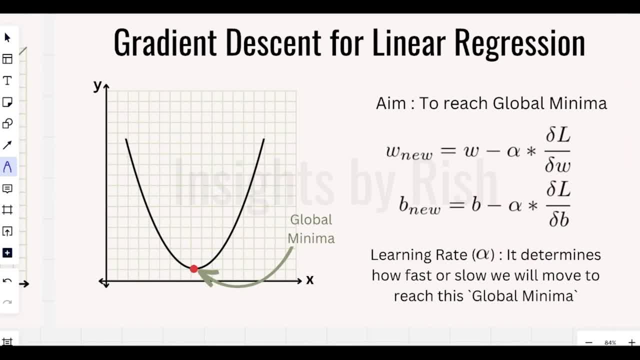 Mean squared error cost function and when you computed the error, you are somewhere here. You are somewhere here In gradient descent. your ultimate goal is to reach here, at this point, which is called as global minima In gradient descent. your ultimate goal is to reach this global minima. 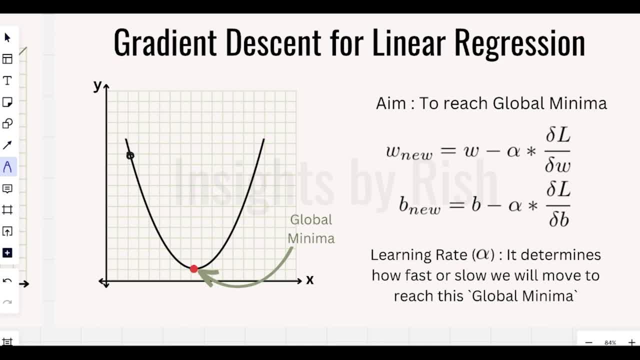 No matter where you are, you can be here, you can be somewhere here, But your ultimate goal is to somehow reach here, because at this point your error is 0,. error is minimum Gradient descent when you plot it in such a way, in a U shape. your ultimate goal is to minimize the error, which means to reach at this global minimum. 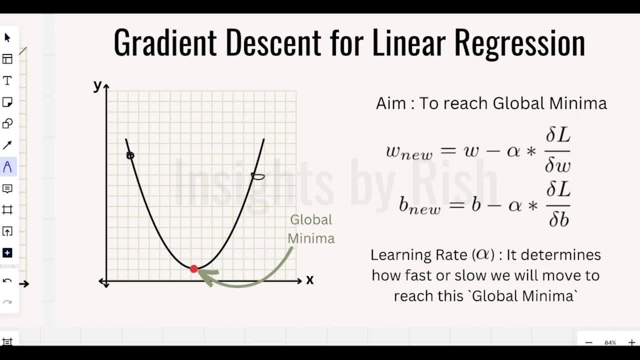 So this is called as global minima minima. to reduce the error, this is the formula for weight updation. now see: first it considered. first your model considered some weight, let's say the weight was w1, and it considered some bias b1. then it plotted the best fit. 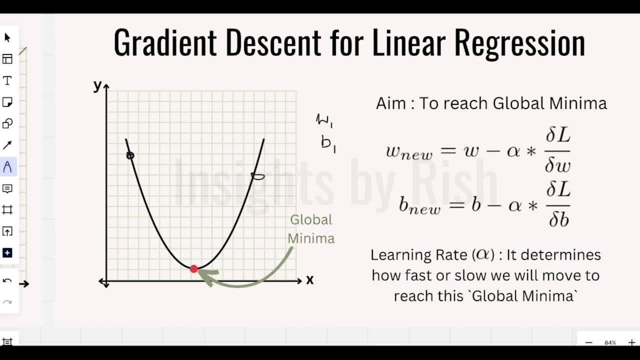 length. then the model again started for second iteration, in which it considered different weight- w2- and different bias as well, which is b2. it will continue it up to some finite iterations and then it will choose the weight and bias. that is plotting your, that is plotting your best fit line, which is minimizing the distance between. 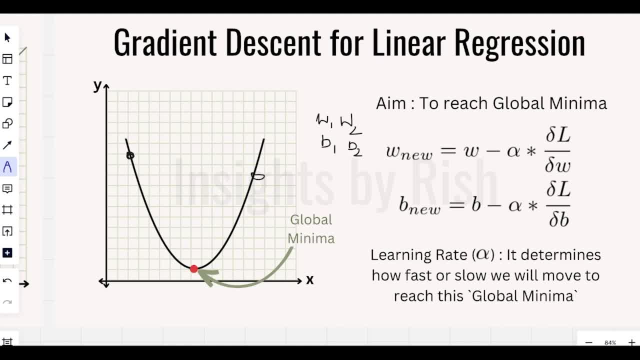 the data points and the line. in this case, this is the formula you can see. your new weight will be your W. it is the old weight. this is your old weight. so you are done. W new will equal to W old minus alpha into. this is the gradient of loss. 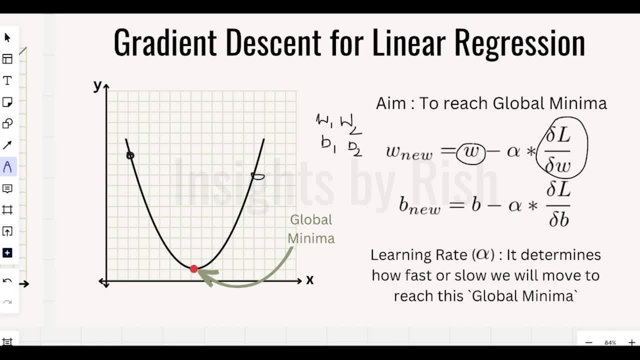 function: gradient of loss function. L is the loss function. that is, mean squared error, mean absolute error. this is the gradient of loss function with respect to change in weight computing. this is again using some chain rule but we won't study this because it has out of scope of our video. 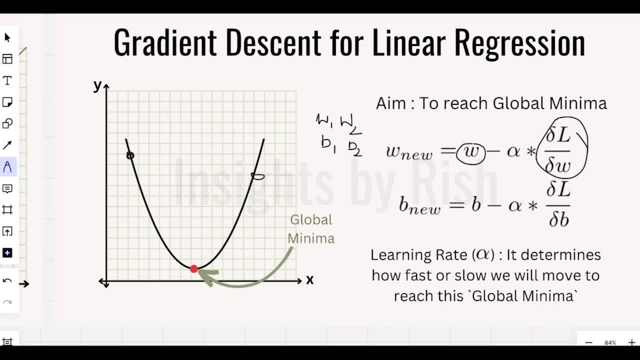 so this is the gradient of loss function with respect to change in weight, and alpha is a learning rate. a learning rate in determined how fast or slow we move to reach this global minima. our ultimate goal is to reach this point, but it depends upon our speed. it depends how fast or slow we are moving towards this point. 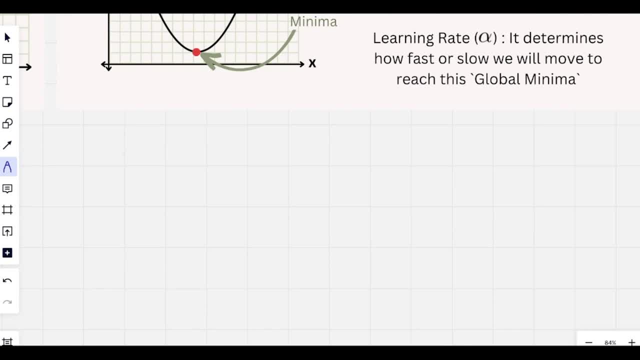 let us understand that. let's say: let's say this is the um, your gradient, descent, and your ultimate goal is to reach. at this point, let us consider that you are having very- uh, small learning rate. let's say you are, your learning rate is alpha 1, which is very small. the learning rate is very. 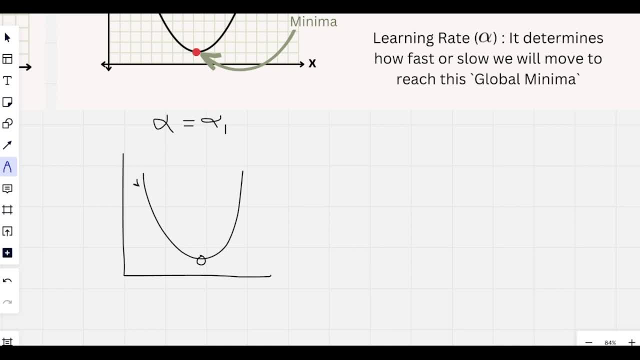 small, which means you will take very small steps to reach this point. very small steps, and eventually you will reach here. but as you are taking very small steps to reach this point, this is a very slow process and in which this means that your model is learning very slowly. 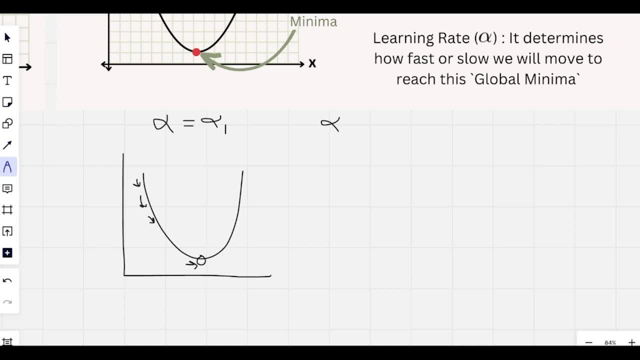 so now you will consider some new learning rate which is very, very large. let's just say that now we are considering some learning rate, alpha 2- and this alpha 2 is very, very large. let's say it is very, very, very large than your previous learning rate, that is, alpha 1.. now, in this case, as our second learning rate, 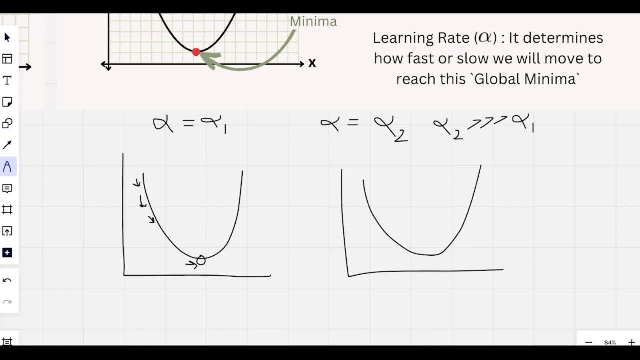 is very large than the previous one. it will take very large step to reach this global minima, due to which what will happen? it will overshoot the condition that is. this is a step. next step it will take here, then from here to here, then from again, from here to here, here to here. 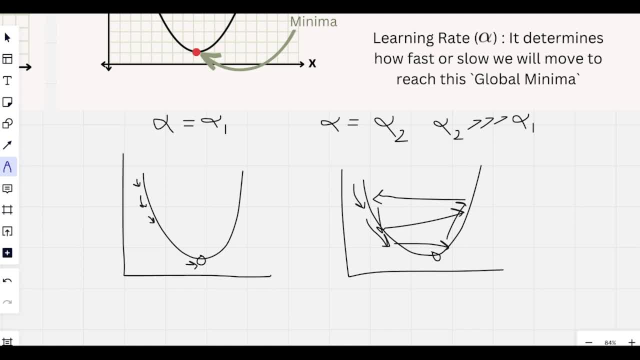 again from here to here. so this means it is just um, moving from here to here, but it is. it isn't actually reaching this global minima, it is overshooting the condition. so when you're learning that is too large, it is just steps taken to move towards this global minima is too large. 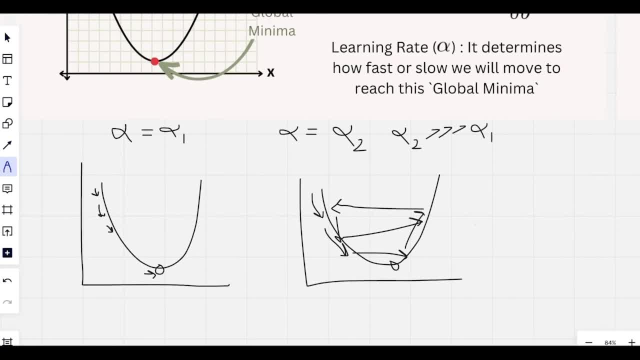 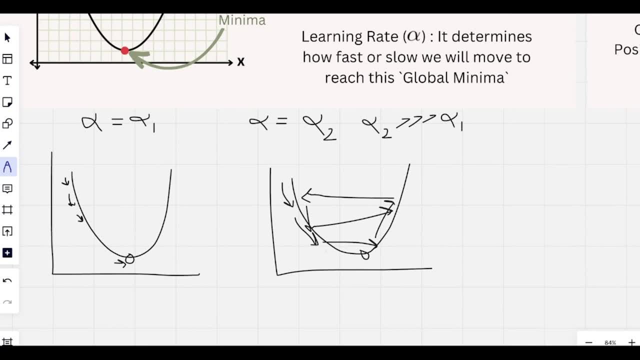 you overshoot the condition. so from both of this with, we came to in conclusion that we do not require a very small learning rate and we don't require a very large learning rate. the learning rate should be adaptive. what do you mean by adaptive? adaptive means it will change depending upon the situation. 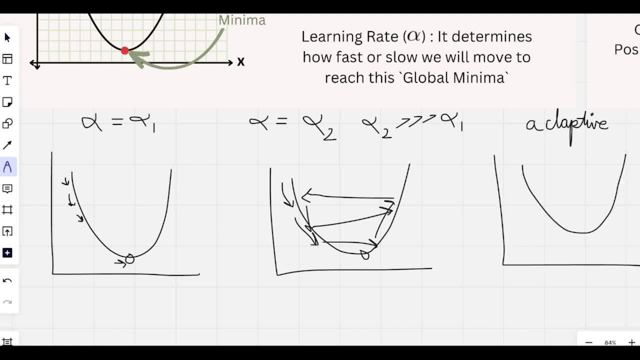 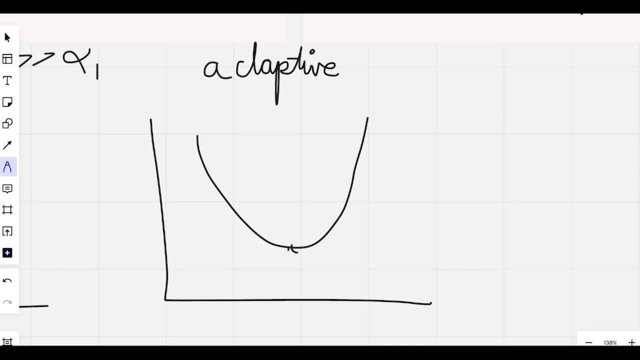 let's say, this is the gradient descent that we have. now we have to reach you. so we have to find such a adaptive learning rate, which means initially it will take larger steps. initially it will take larger steps, but as you approach to this global minima, as you approach this global minima, 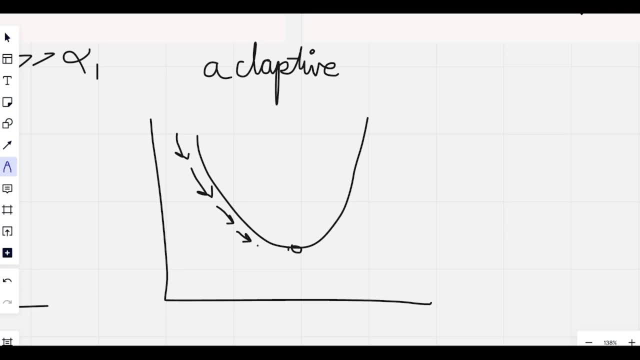 the learning rate will be reduced now. it will start taking smaller steps in order to prevent overshooting the destination. this is the adaptive learning rate, in which initially, you are taking larger steps. that is, your learning rate is large initially and as you are approaching this global minima, you reduce this learning rate. 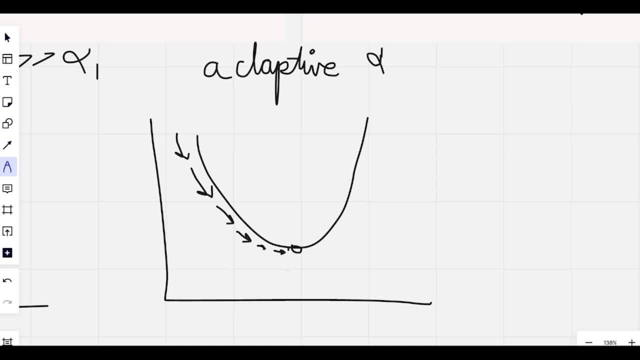 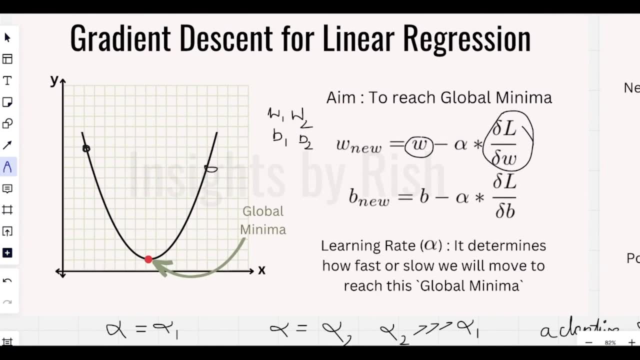 where you take small steps in order to reach the global minima without overshooting the condition. so that's the importance of our learning rate. now, same formula is applicable for bias as well. your new bias is equal to old bias, minus a learning rate into the gradient of loss with respect to change in bias. 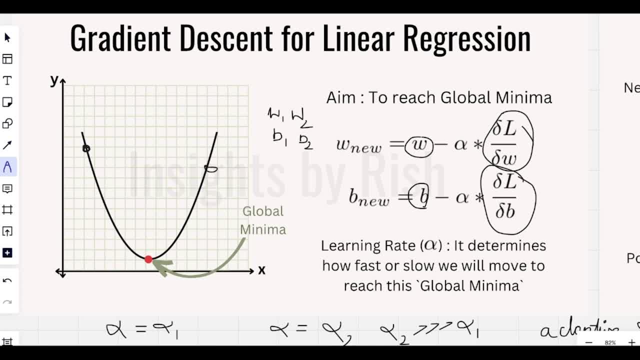 now we won't go into detail of this uh formula, because that will be out of the scope of this video uh, but these are the formulas that you use to optimize the way you are learning weights and biases in order to reach this global minima. now there are two cases here. let us say that, initially, when you computed your 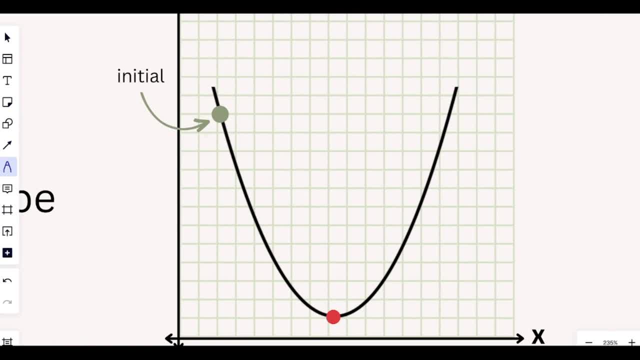 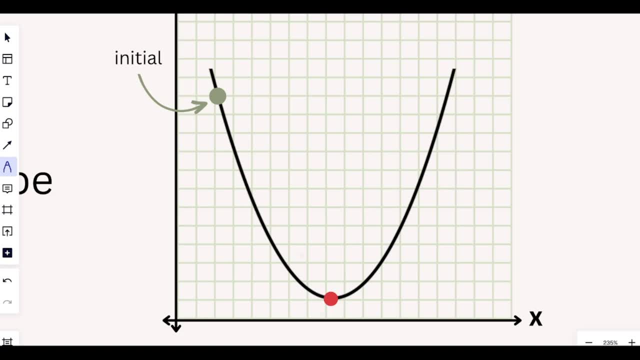 cost function. uh, your mean squared error. you are somewhere at this point, which means now you have to minimize your cost error and you have to reach it at this global minima. so at this point your slope is negative. you draw the tangent, you draw this tangent and when you take the slope it is a negative slope, as i 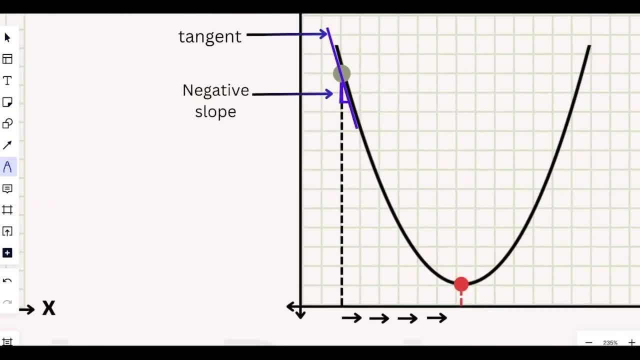 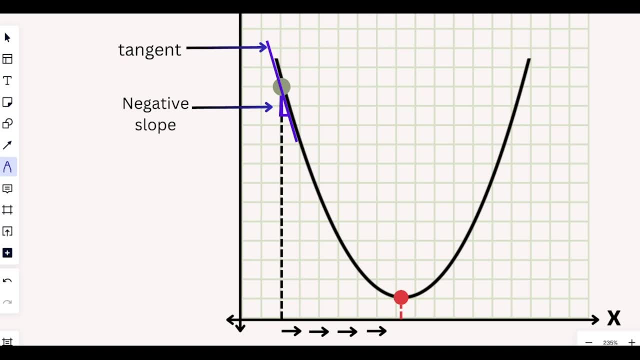 have drawn here. you draw a tangent at that point and you take the slope, which is a negative slope when you plot that onto this x-axis. this is where you are now. in order to reach the global minima, you have to move in a forward direction here, while in a second condition, in the second 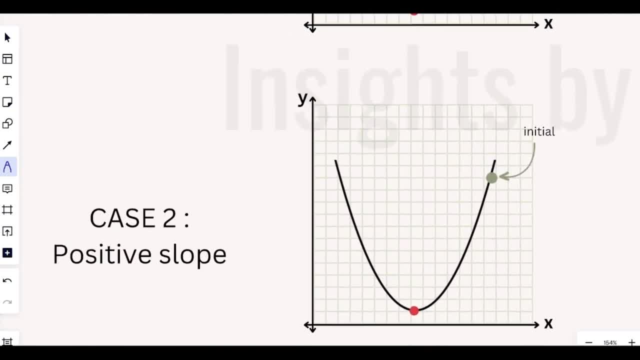 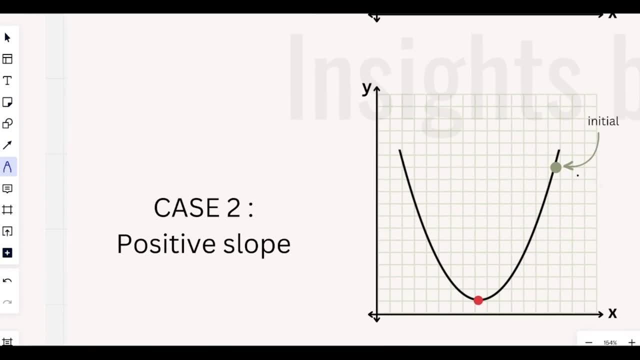 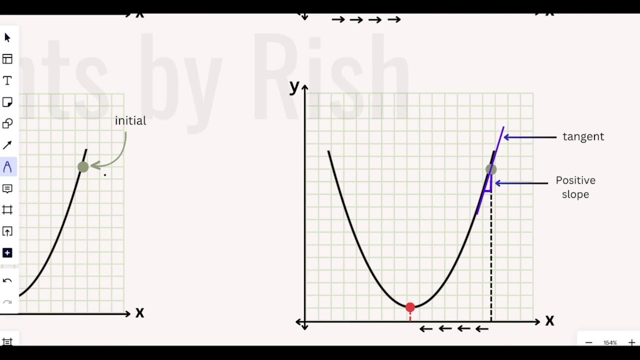 condition. let's say that you computed your mean squared error and you are somewhere here. now, in order to reach the global minima here, you have to move backwards, because when you will take a tangent here, this tangent, and when you will compute the slope, it will be a positive slope. now, when you plot that line on your x-axis, 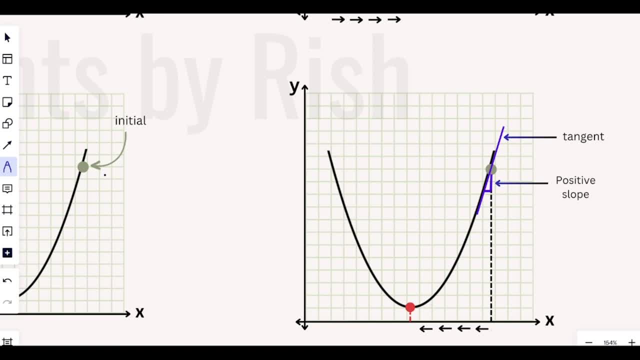 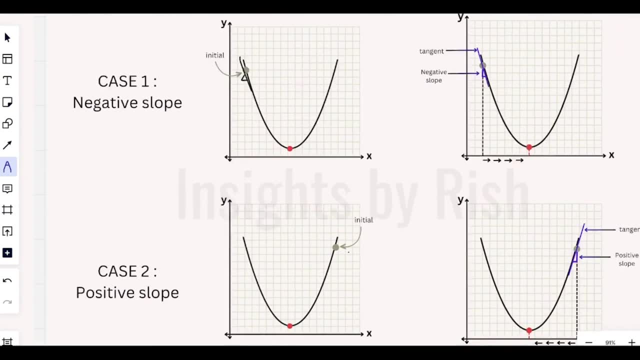 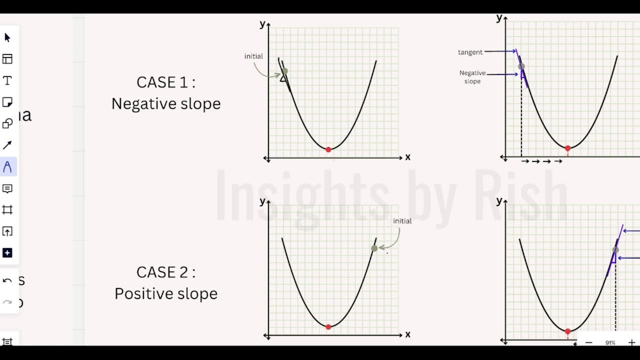 you have to move backwards in order to reach this global minima. so these are the two cases of gradient descent here. this was the basics of gradient descent in linear regression. so gradient descent is in: uh. in short, it is a strategy to optimize your weights and bias, optimize your loss. here you are optimizing your features. 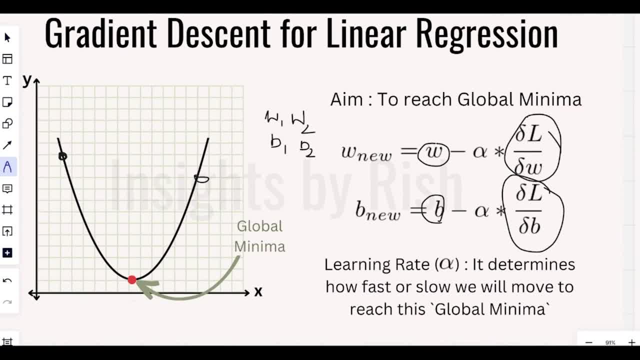 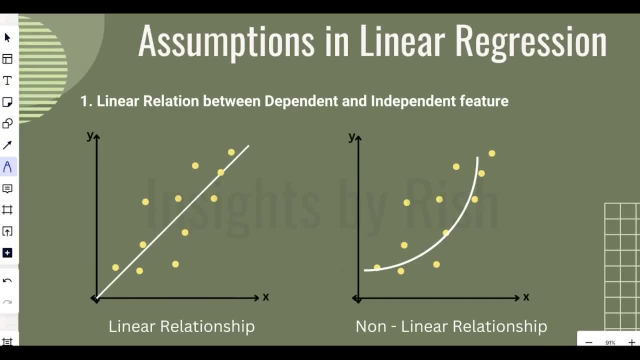 this weights and bias in order to to reach this global minima, which means you are trying to reduce the error and increasing the accuracy of the model. now let us understand the assumptions in linear regression. while performing the linear regression task, we assume some things, and that are. the first one is 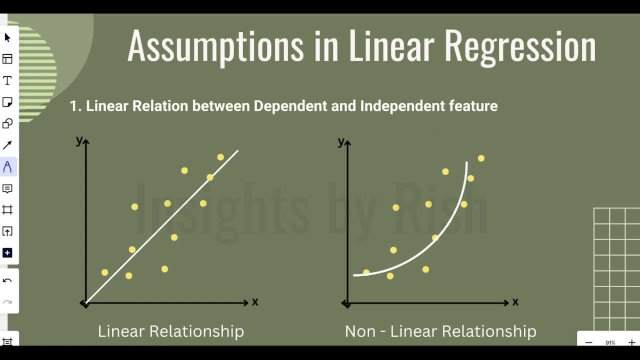 linear relationship between dependent and independent variable, as i said in the initial stage, that we assume that as the value on the x is increasing, the value on the y also increases. that is when your number of hours you study increases, your marks also increases. so that's a linear relationship. while this is a 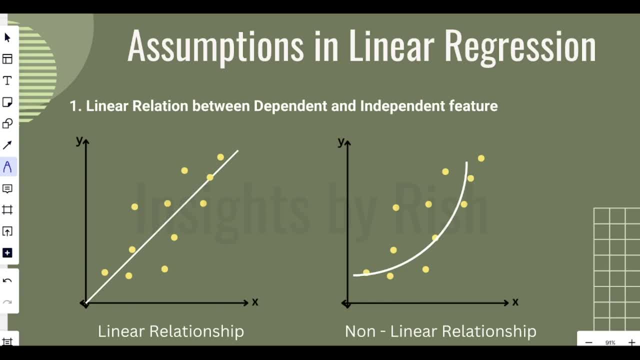 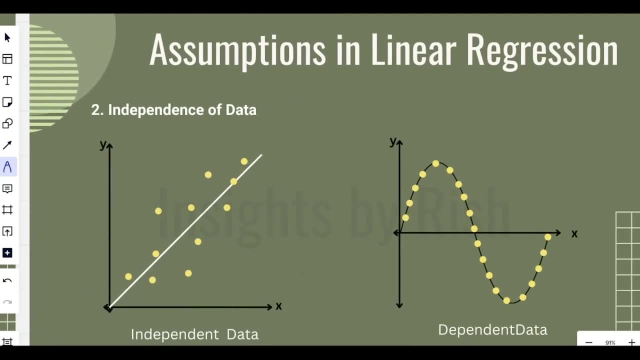 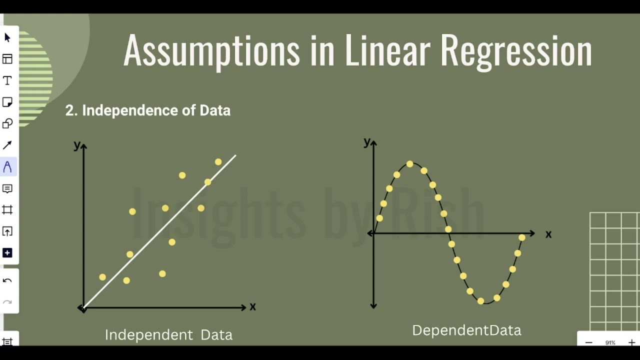 non-linear relationship and we are assuming that our data is following this linear relationship while performing the linear regression. the second assumption that we make is independence of data. by independence of data, i mean is like: here, the data points aren't dependent on any uh on each other. here every data point is. 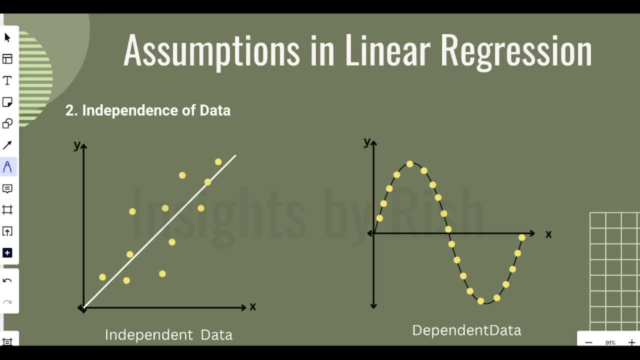 independent from every other data point, while in dependent data point, your current data point is dependent on its previous data. let's con. let us consider the example of uh patient. the patient's today's data, that is, uh, his, how well he has recovered, how he is doing- will be dependent on his previous. 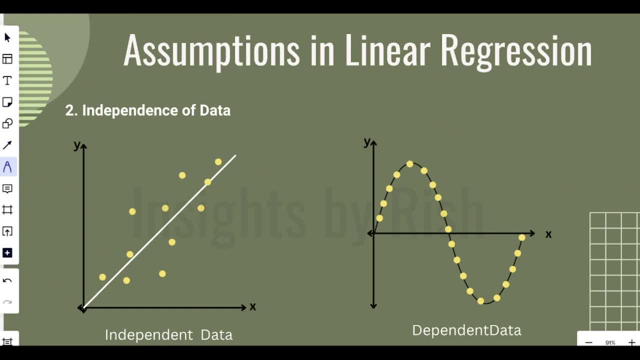 data. that is the medication that he took yesterday, the treatment that he took yesterday. depending upon that yesterday's data, his today's health will will be decided. so here, your data is uh dependent on the previous data as well, which is a time series data, and such a data is called as dependent. 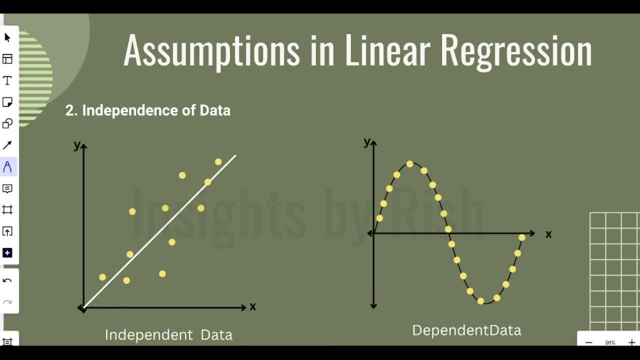 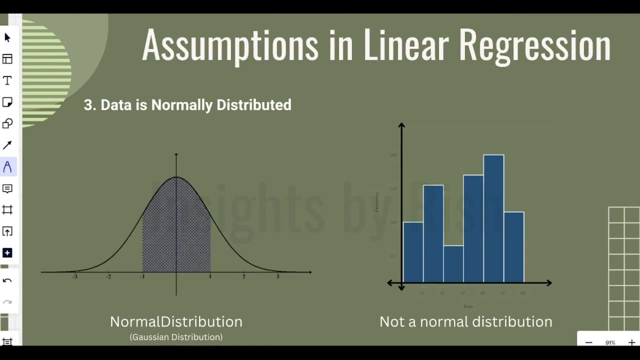 data. so, while performing linear regression, we assume that our data is independent. that is, it is uh. there is no multicollinearity and every data point is independent from every other data point. the third assumption that we are making is our data is normally distributed. this is a. 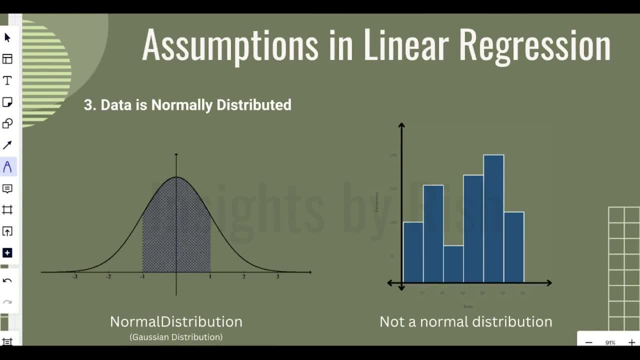 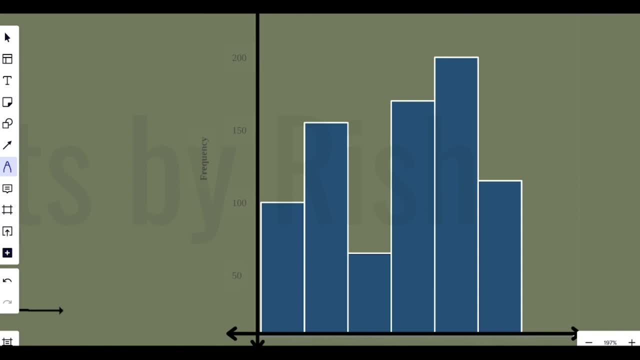 normal distribution, uh, which is also called as gaussian distribution, and this is not a normal distribution. this is uh. in this, you can see, the distribution is somewhat like this and you reach here, from here to here and then again from here to here. so this is not a normal distribution, while your normal distribution is always. 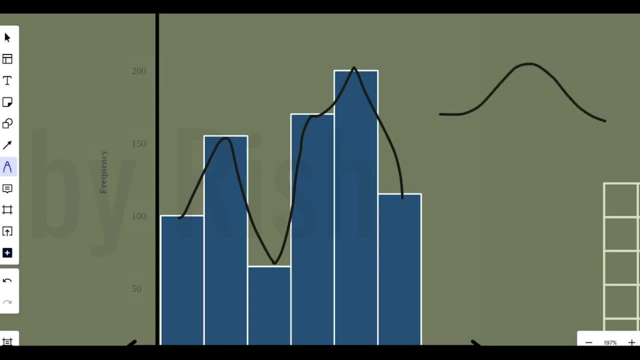 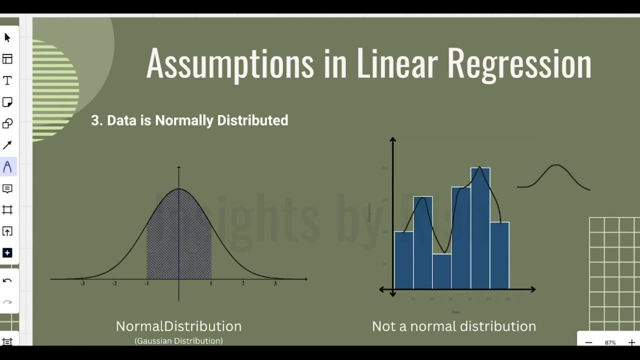 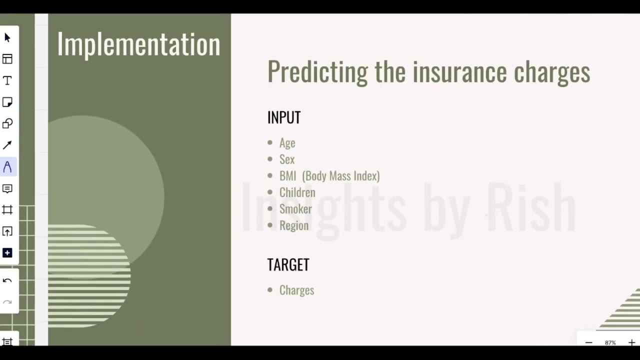 in this fashion: it increases at some point and it again decreases. so in linear regression, we assume that our data is normally distributed in this way. now, as we have covered all the concepts of linear regression, we will see some implementation for implementing linear regression. uh, we will be having this data set. 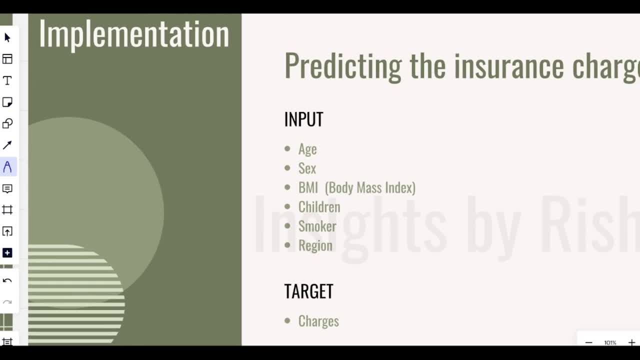 uh, where you are, where you have this input and you have to predict the insurance charge. so in input you have the age of a person, the sex, that is, the gender of a person, the body mass index, the number of children he or her- uh, they have a smoker- and the region feature. 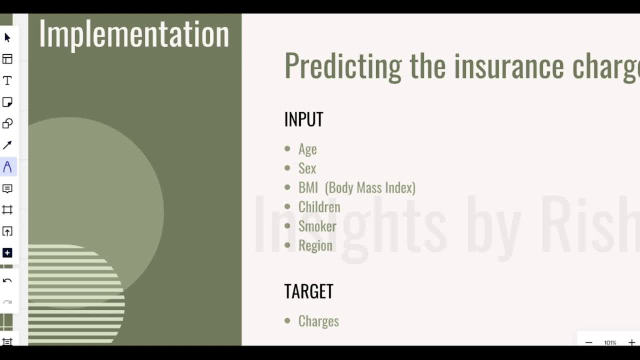 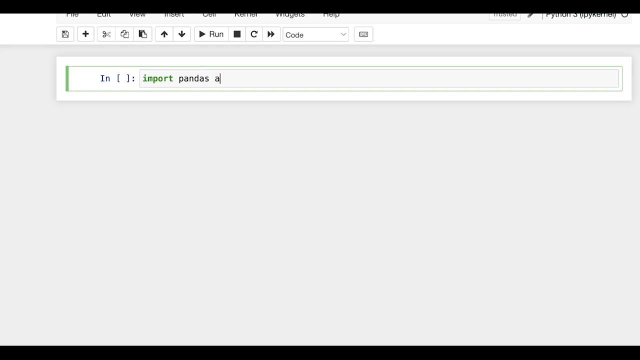 and, depending upon all these input features, you have to predict the insurance charge for that person. this is the example of multiple linear regression, where you are having multiple input features. so let's start coding. let's start with coding. we will import the pandas library and we'll import warnings to ignore the warnings that the jupiter lab gives us. 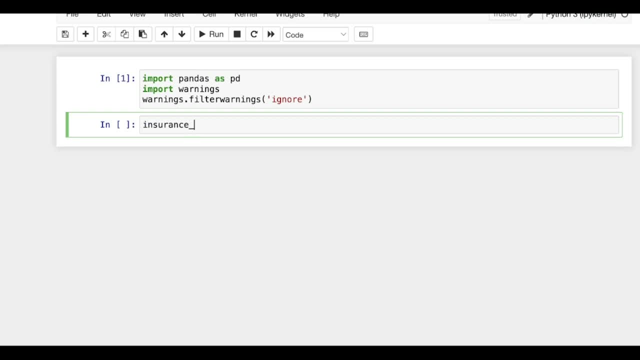 now let us load the data set. insurance df is a data frame in which we load the data set. this is the path on which the data set, on the on which the csv file is stored. let's display it. this is our data set. uh, you have eight. 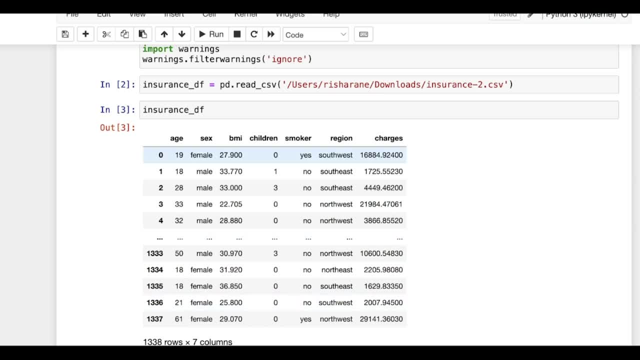 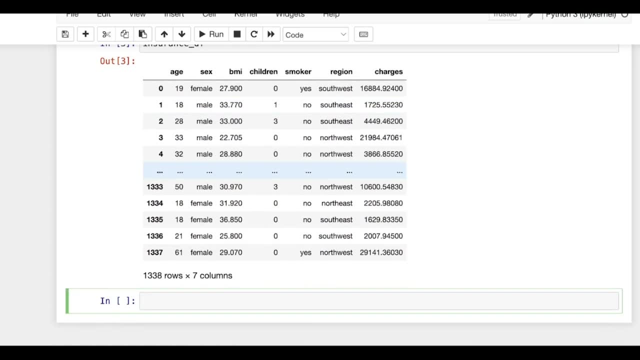 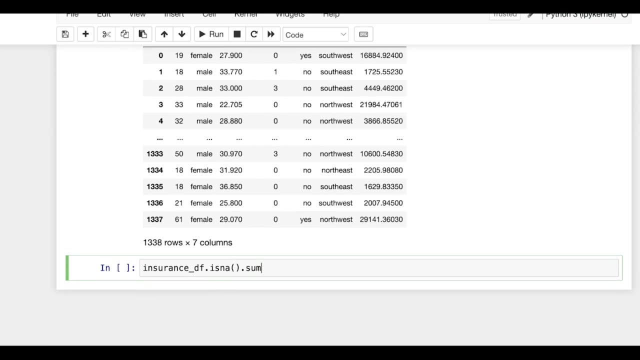 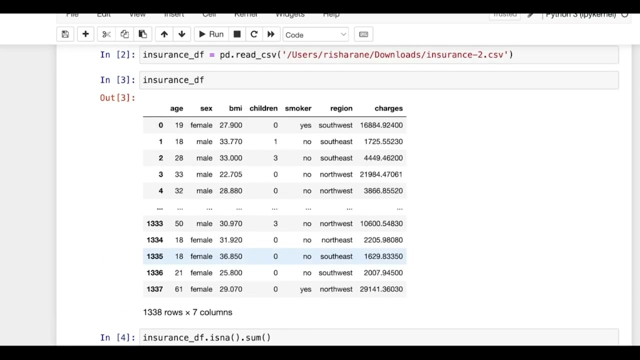 sex, bmi, children, smoker region and depending upon all these input features. so you have to predict this charges. we'll start with data cleaning. let's check whether it has any null inputs or empty values. as you can see here, we don't have any null inputs, so we can directly start with data processing. 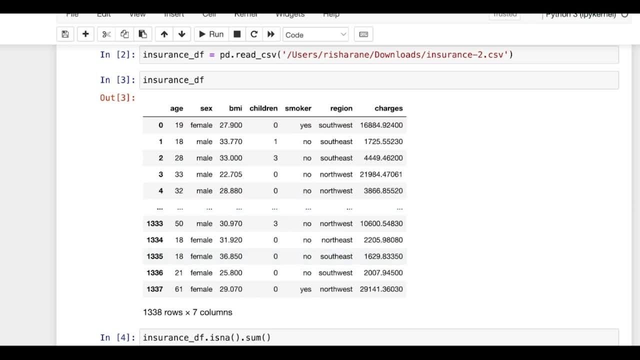 now in this data set, as you can see, there are several categories. we have some categorical features like sex regions, smoker, so these are the string values. these are the categorical features and machine learning cannot handle such features. machine learning only requires the values in numerical format, so we need to convert these features. 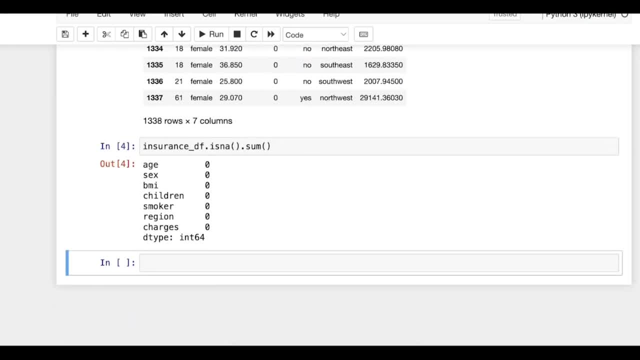 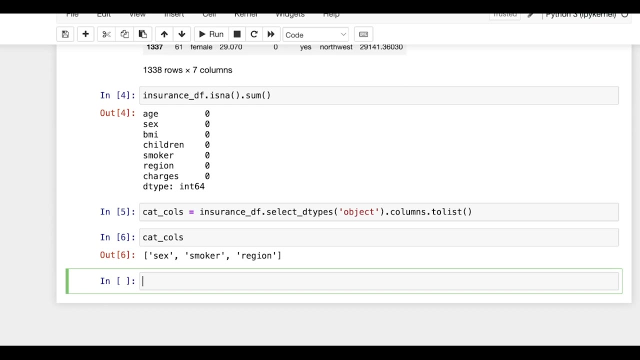 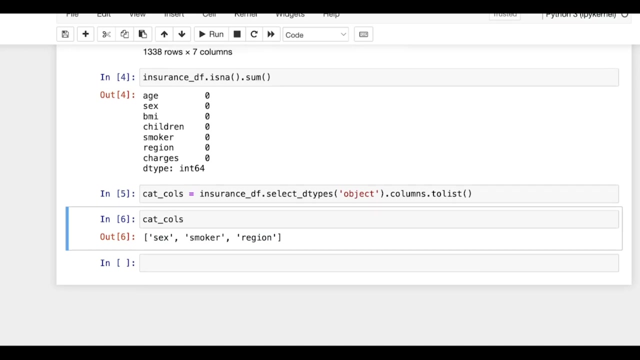 into numerical format. let's start doing that. let us take all the categorical features. let's display so you can see: these are the three features. that contains the categorical values. now we will convert this categorical values into numerical ones using the sk learn library, one hot encoder. so let's import that. 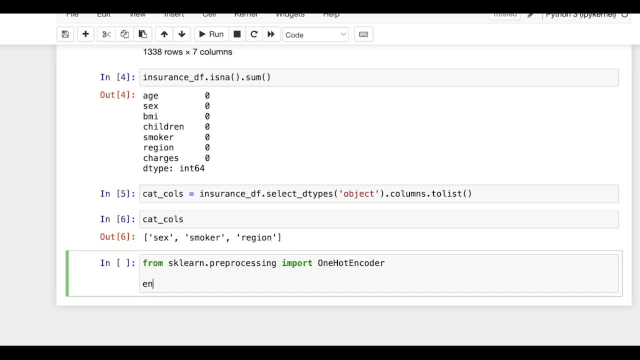 we will create a new code. we will create an object of that encoder is an object of one hot encoder module parse is false and we'll ignore the unknown values. so handle unknown, ignore. now we will fit this categorical features into this encoder encoder dot. fit the categorical features of this insurance data frame. 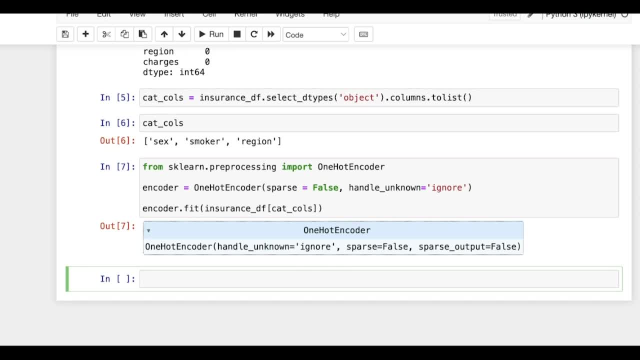 so now we have successfully fitted, now that we are creating new columns with the numerical attributes, um, we need new column names for it. for that, what we will do is we'll create a encoded calls. we will use the function of an encant encoder, which is get, get feature names out from categorical columns. 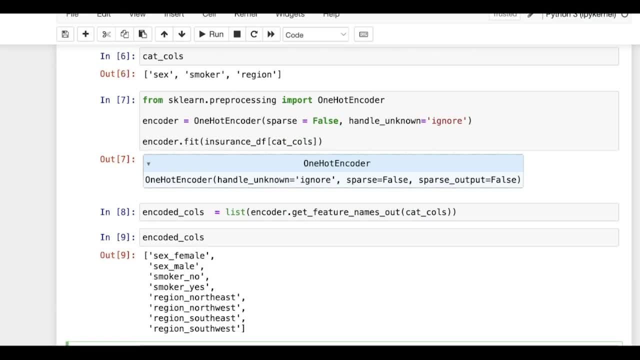 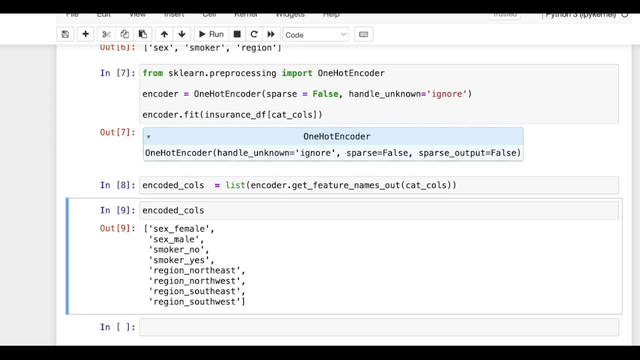 let's check, so test the함 uh column names that we will insert it in our data frame. so it created a new column for every attribute, like female, male, no, yes, and it will consist of values in a combination of zeros and ones. let's add this into our data frame. 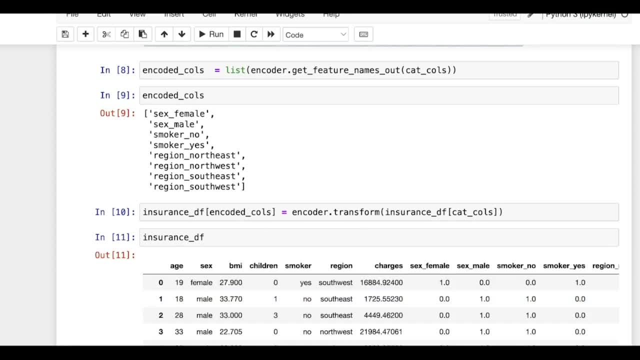 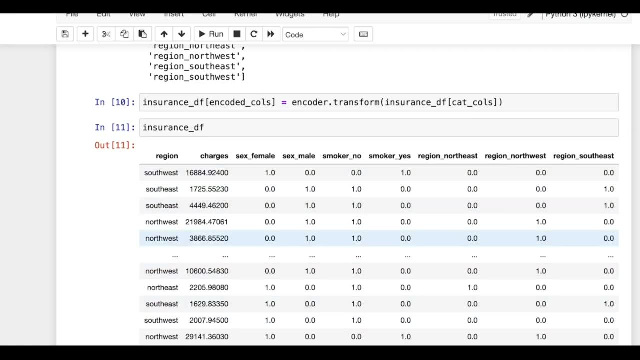 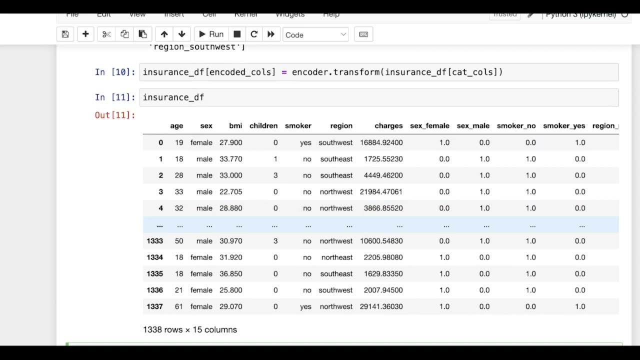 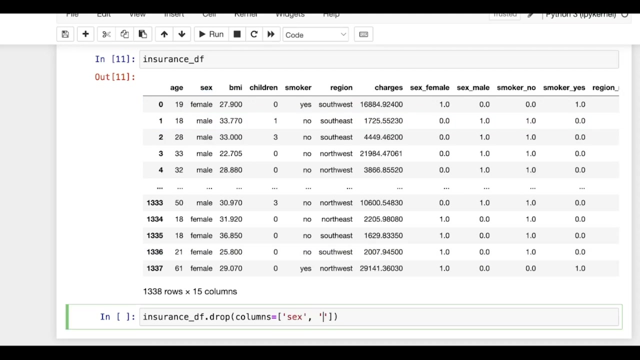 let's check our data frame. so this is the data frame. the new columns are added. every attribute has turned into a new feature, so now we don't require this original categorical column, so we'll delete them. we don't require this text column. then smoker and region. 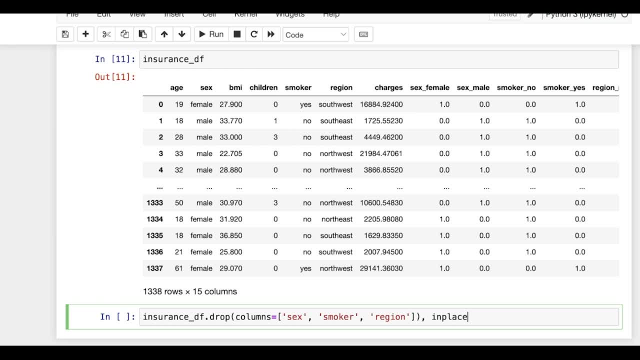 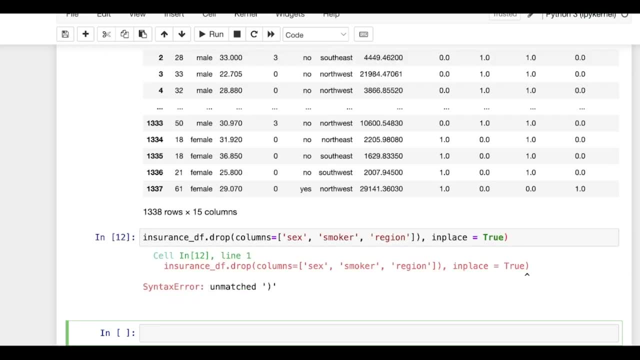 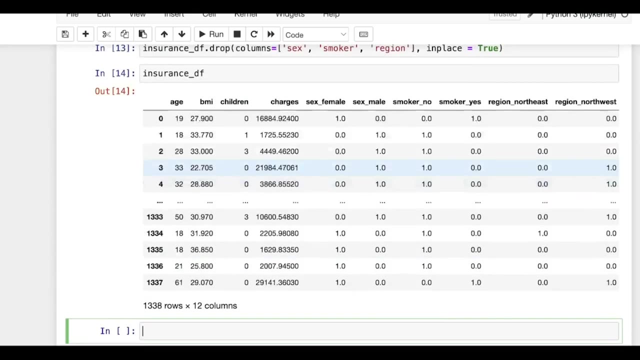 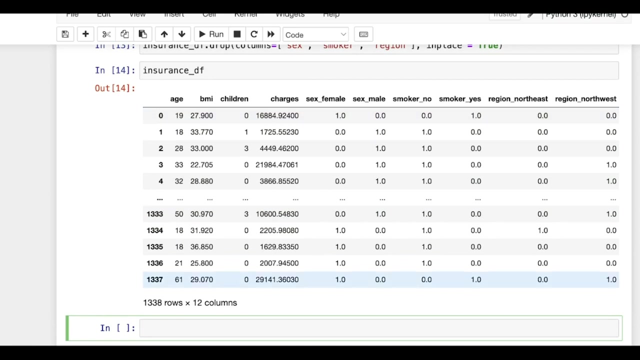 in place. true is used to make the changes permanent changes. if you don't use them, the changes will be temporary. let's display it so. now we don't have this categorical column. all the data that we have is in a numerical fashion. now, as we can see the day, every column has a is on a different scale. 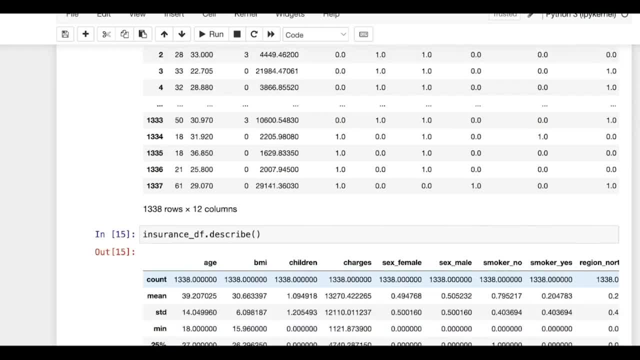 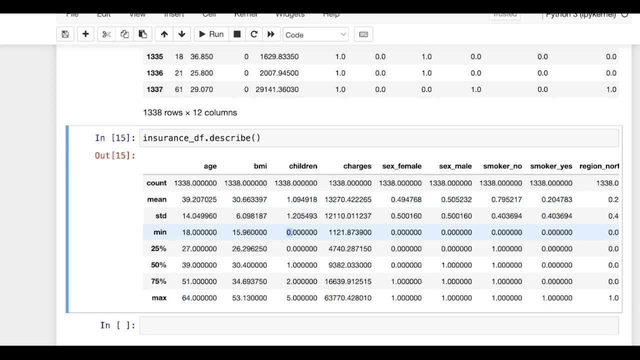 let's, let's check this: when you check the h column, the minimum value is 80 and the maximum is 64.. for children, the minimum value is 0, maximum is 5. for charges, it is 1000, uh up to 63 000. so for every column, uh, the scale is different. so before training the model we need 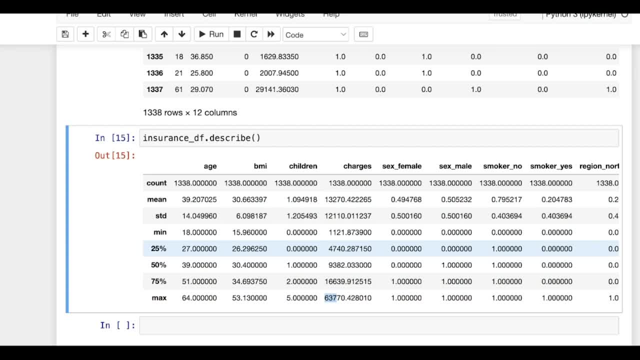 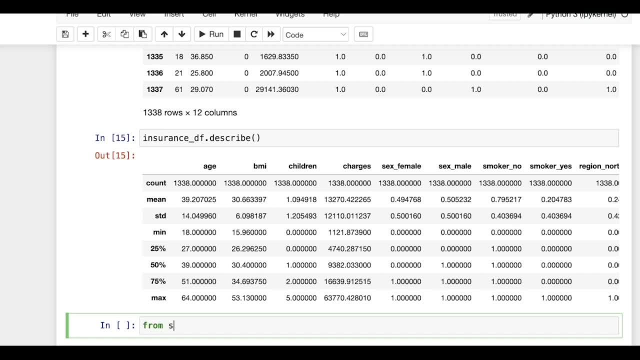 to bring the scale of all this column onto one standard scale, and we will do that using the min max scalar library, which is used for data normalization. so from sk learn dot pre-processing. so from sk learn dot pre-processing. so from sk learn dot pre-processing. import: minmax scalar. 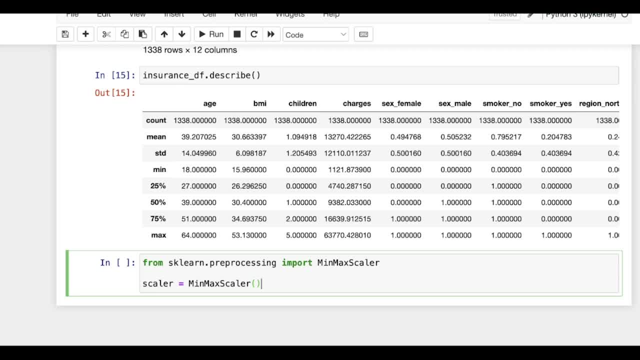 creating the object of minmax scalar, which is: uh, this is an object of minmax scalar module and we will fit our entire data frame into it. okay, let's. before doing this, let us divide the data frame into the input features and the target column, let's say x is our input feature. 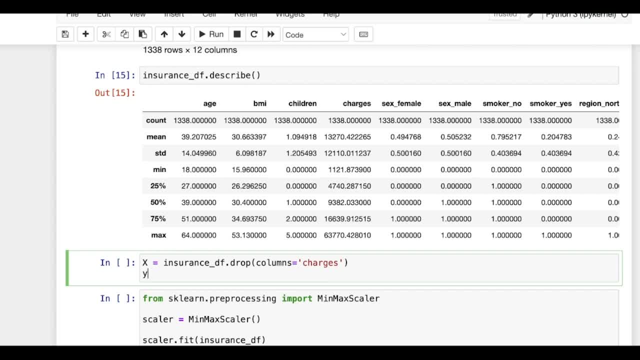 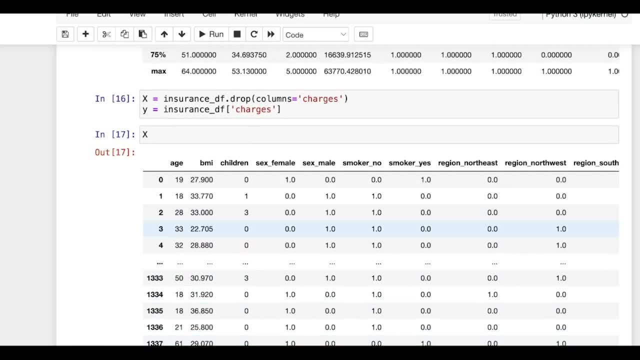 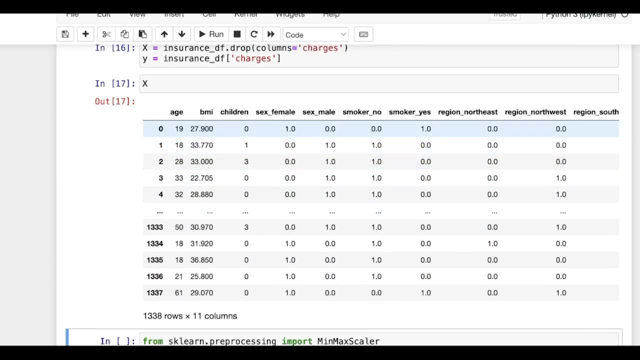 and the target feature will be the charge. as you can see, this is will be our input here. we don't have the charge variable. the charge feature is our target feature here. we don't have that. we are going to predict that now. we will scale the whole input data using the minmax scalar, the minmax 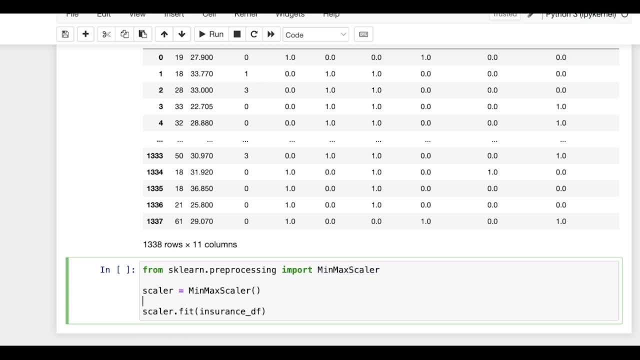 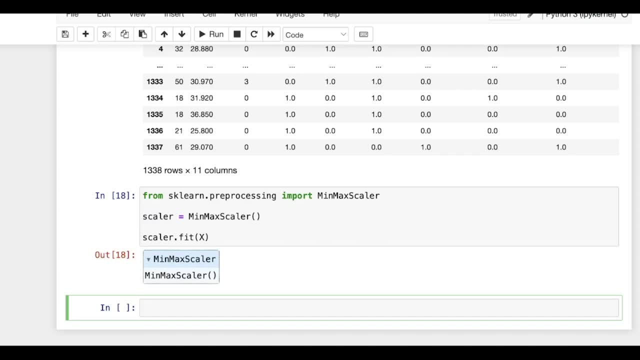 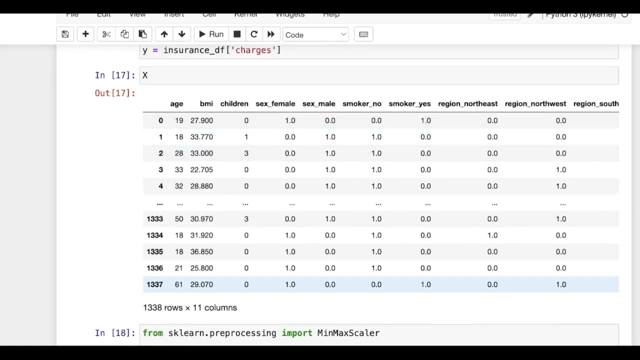 scalar basically scales it between 0 to 1.. we'll fit it into the input one basically scales it between 0 to 1.. we'll fit it into the input one now. let's transform it now. when you display, see here the data was on different scale for every column. 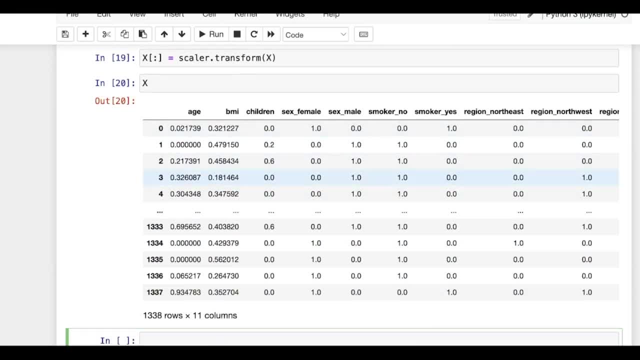 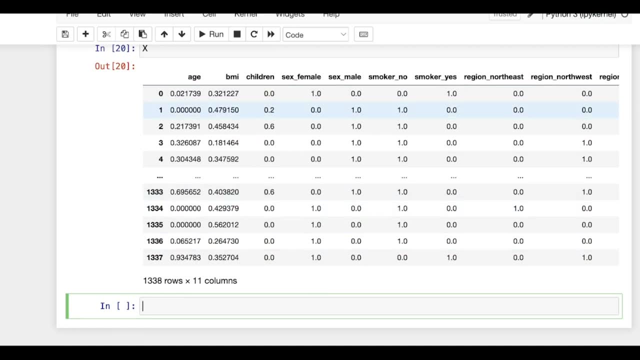 here for every column, the data is between 0 to 1, so that we have scaled it between 0 to 1 using the minmax scalar library. now that you have scaled, we will do the trend test split. basically, we are dividing this data set into some training set and a testing set. 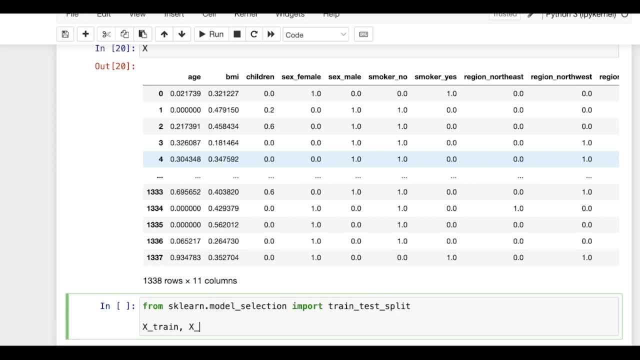 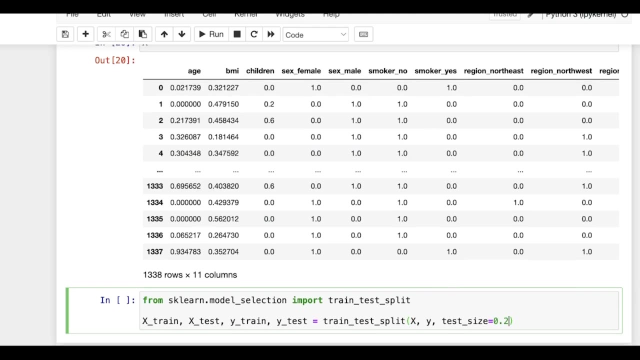 using the minmax scalar library. now let's see how we do it: input, data set feature and test size. test size is 0.2, which means 80 data will be into the training set and 20 data will be into the testing set. and random state is 42, which means we will get same data for every iteration. 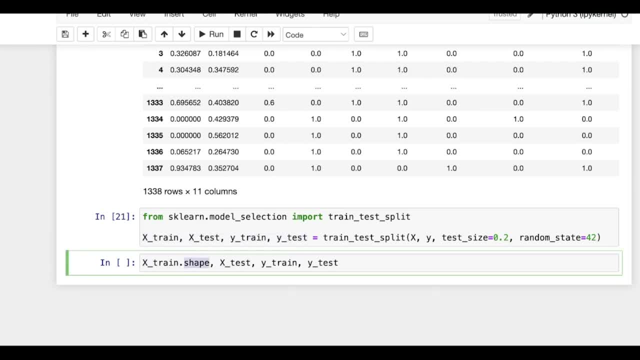 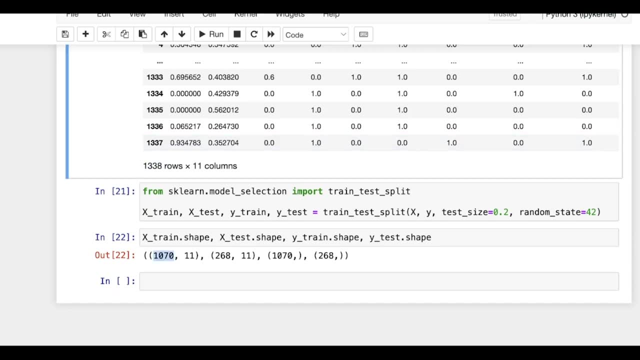 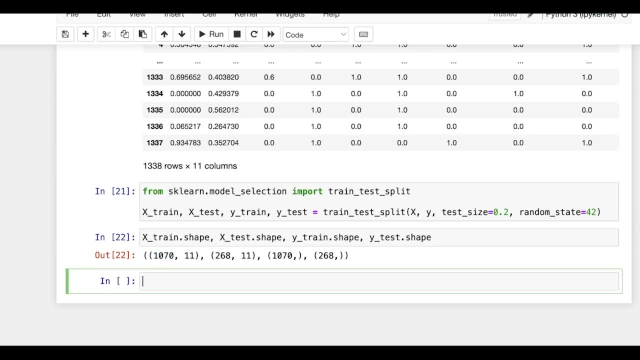 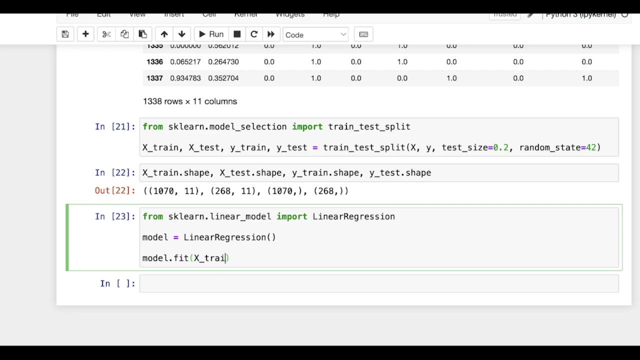 in testing set. now let's train the model. so from sklearn dot linear model we will import linear regression and, creating the model that is an object of linear regression class, we will fit it into our x train and train, y train. that is our training data set. so we'll fit this training and testing data set. sorry, training input and training target data set. 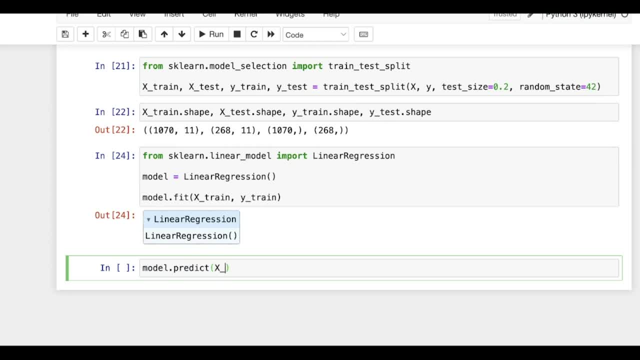 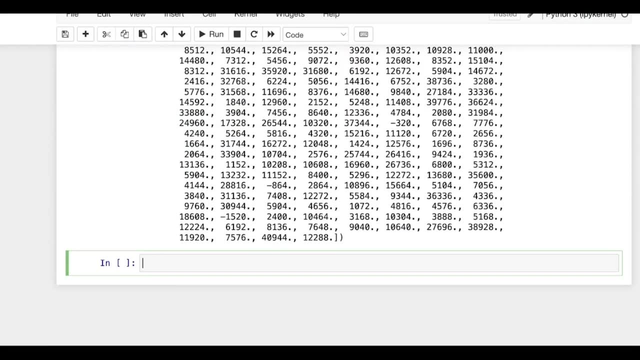 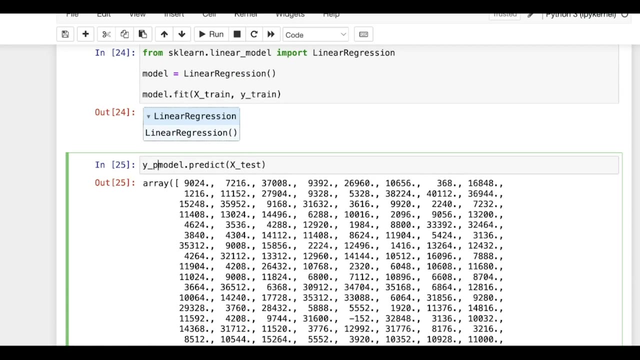 now let's do some prediction. let's pass this testing data set. so okay, what were the actual values for this? the actual values were stored in the test data set: y test. these are the actual values. let us store this into some y predicted. these are actual values and let's check the predicted values.